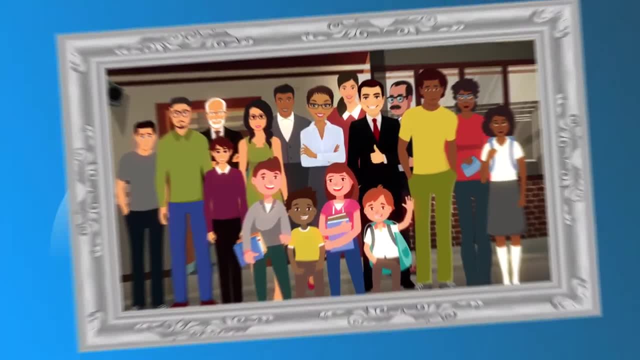 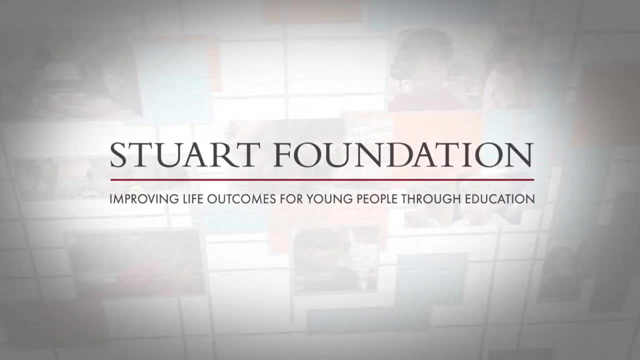 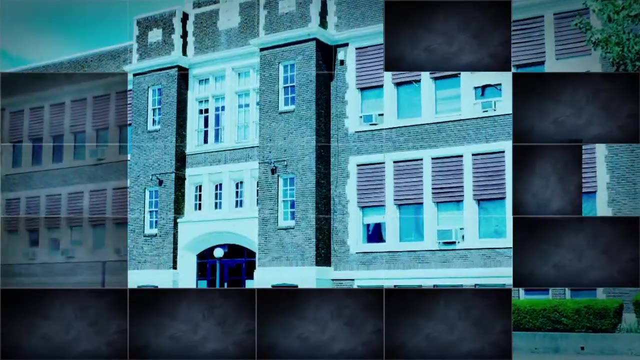 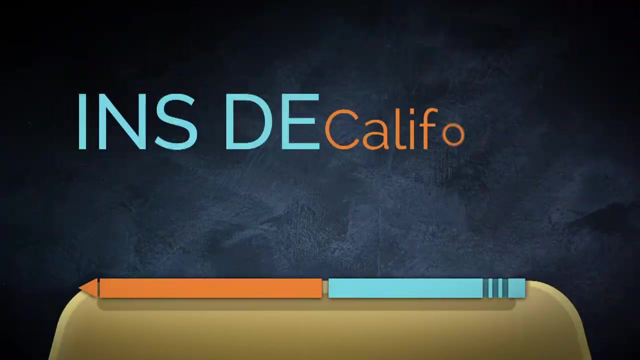 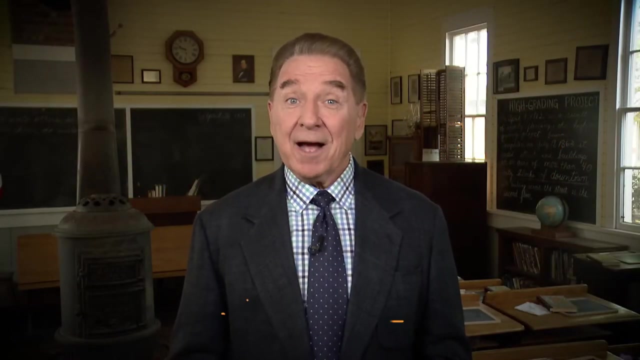 and active parents. every public school student can realize their dreams. The California Lottery: Imagine the possibilities. The Stuart Foundation, Improving life outcomes for young people through education. Welcome to Inside California Education. I'm Jim Finnerty. We start at California's state capitol, where students at one 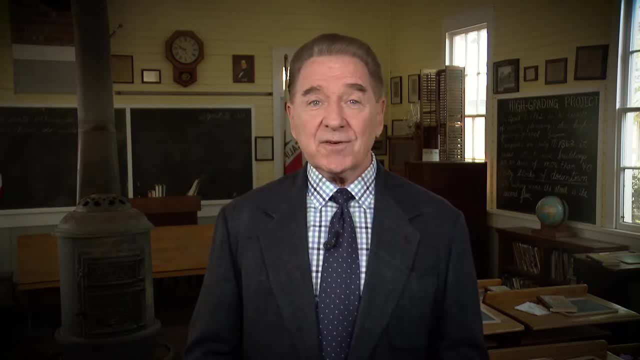 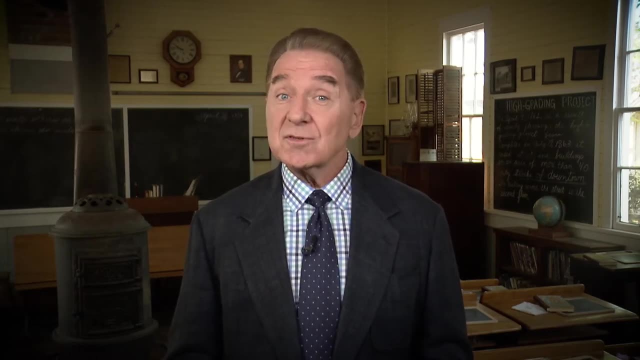 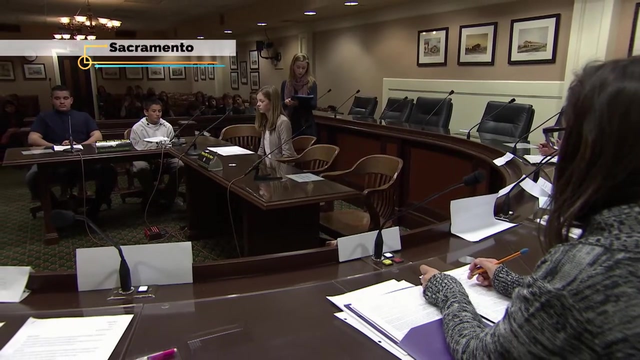 high school are participating in an intense four-year civics education program. It's called Civitas and supporters say it's helping to create a new generation of civic leaders. Now I understand, from a logical perspective, that schools cannot simply decrease the tuition or not increase at all for a limit. 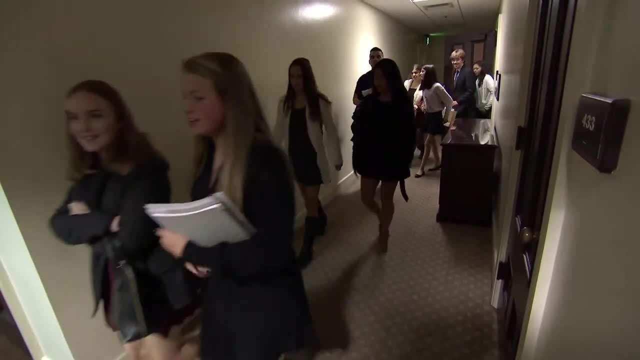 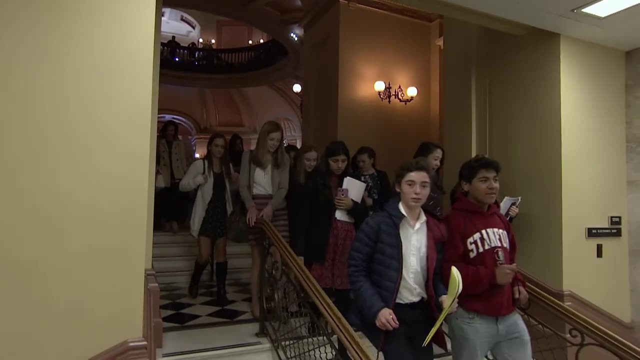 of 5% increase every year. These are the halls of the California State Capitol And these are the young men and women who are building the knowledge and honing the skills to someday work here. Hello, I'm Haley Phillips. As a student, I believe there should be no. 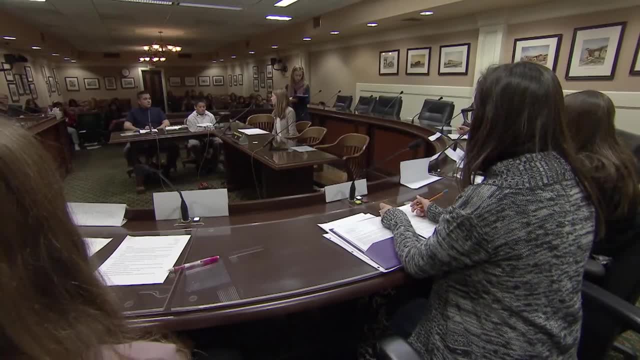 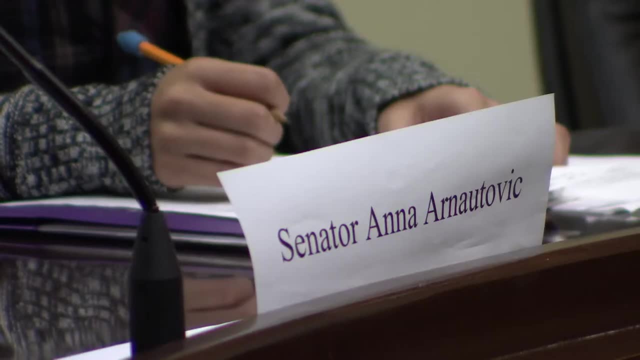 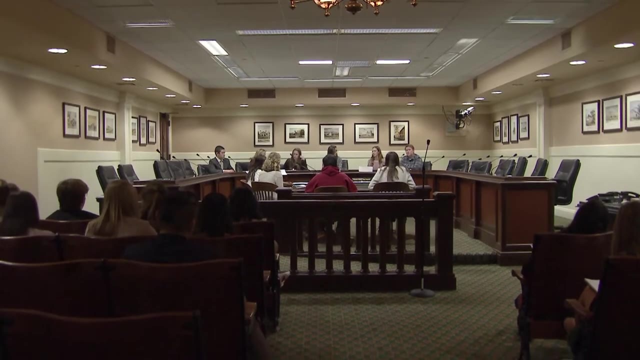 tuition increase. On this day, students from the freshman class at Sacramento's Rio Americano High School are holding a mock senate hearing in an actual hearing room at the capitol. They're in the first year of a program called Civitas, a four-year focus on civics education. 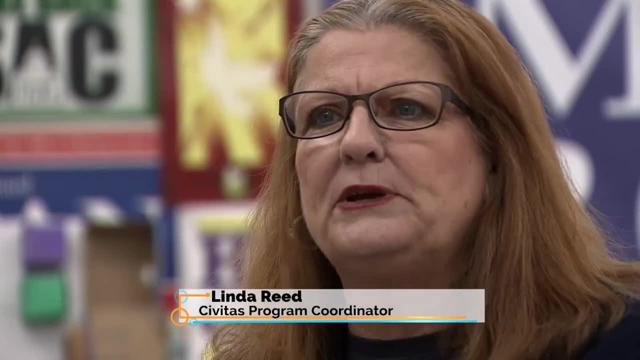 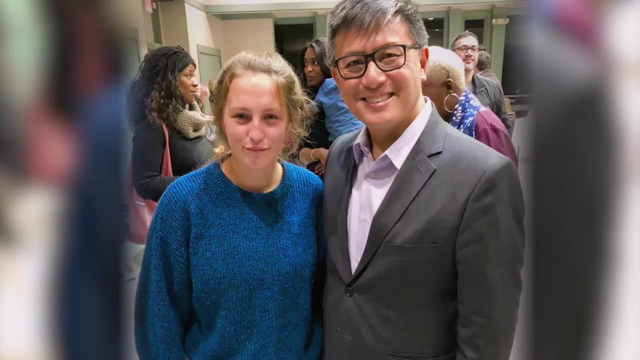 Civic education to me is not the same as taking your government class. Your government class should be there and you should understand how the apparatus of government works. But this is more about activism and getting kids to do community actions You should also be involved with well. 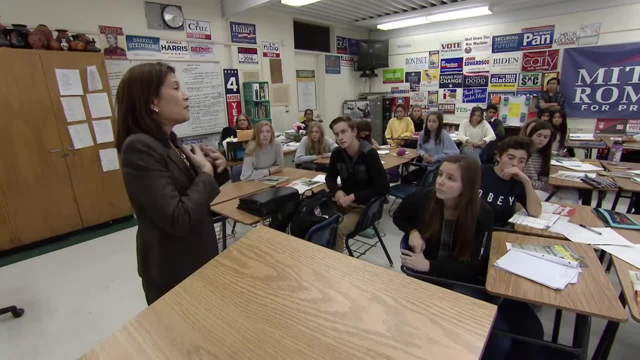 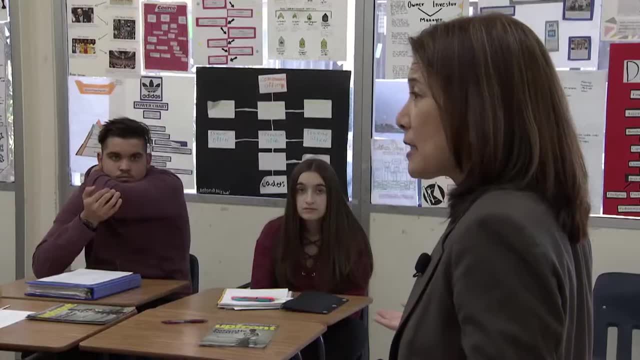 who are your politicians and what are the things that are on the ballot? I'm a state court judge. Immigration is not anything that I do on a regular basis. Many in education and government say civics learning is gaining momentum amid a growing recognition of the 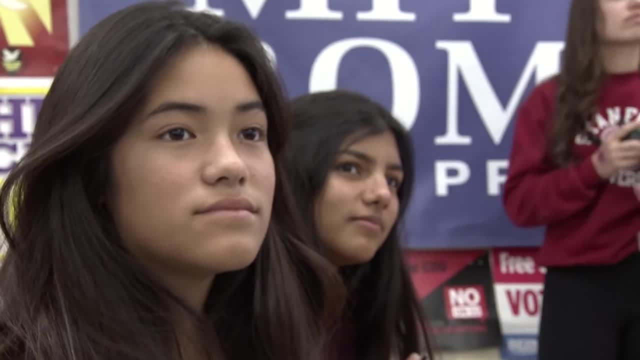 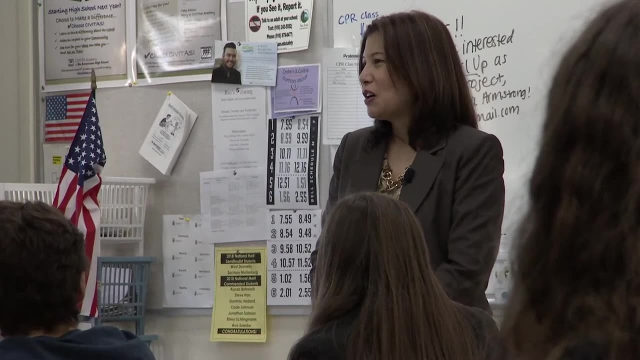 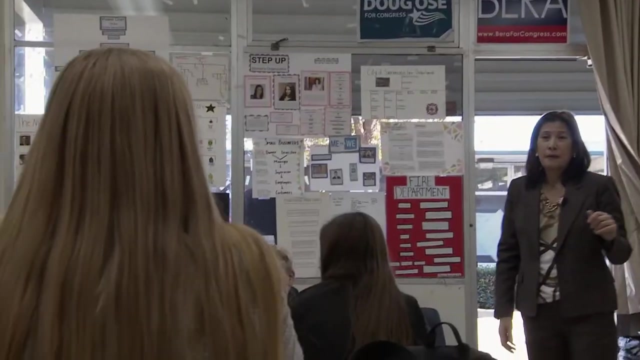 importance of better preparing the next generation of leaders. One of the state's biggest advocates is California Supreme Court Justice Tawny Cantil-Saka'ui, who co-created a statewide steering committee for civic engagement and education. in schools, Students have questions that I think are well beyond their. 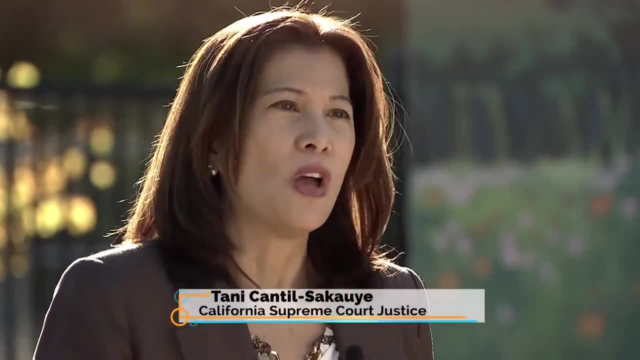 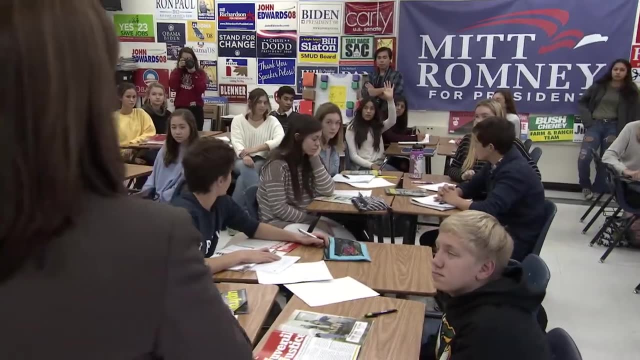 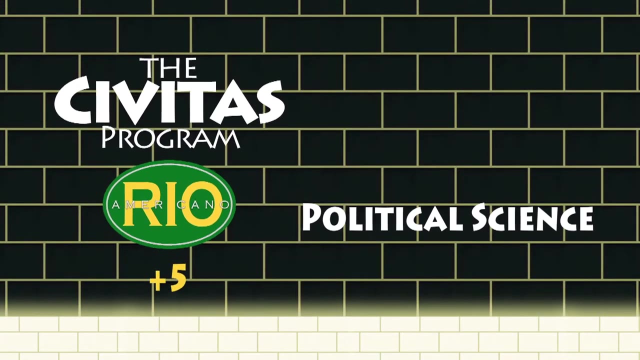 years about what their future looks like and how could this be happening now and what makes that so and what is that? And so they're thinking about leadership and decisions they would make and choices they would make. The Civitas program at Rio Americano includes a rigorous 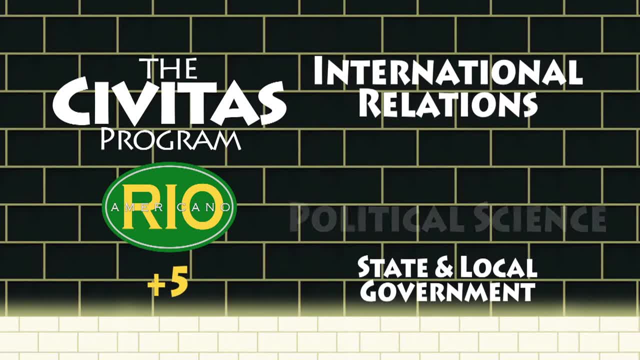 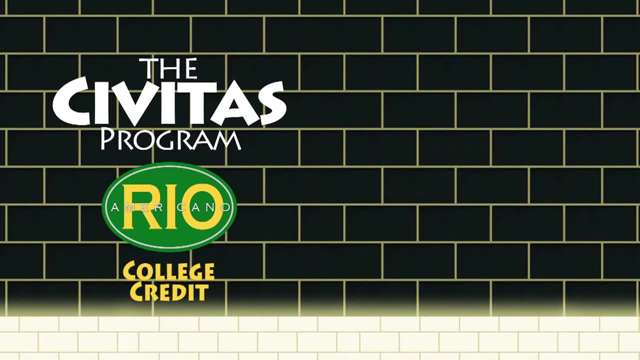 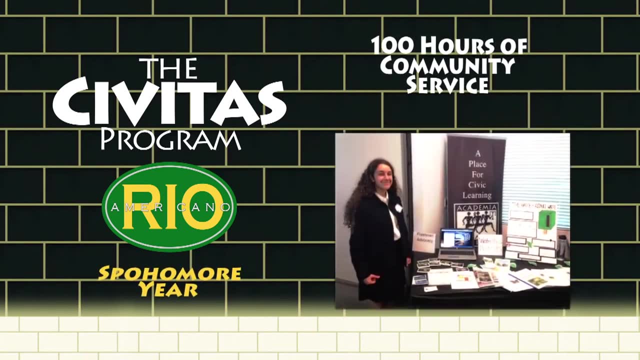 curriculum of academic and engagement activities. Students are required to take five extra courses throughout their high school years that can translate to college credit. Their freshman year focuses on national, state and local issues. During their sophomore year, students complete 100 hours of community service, from working on a campaign to volunteering. 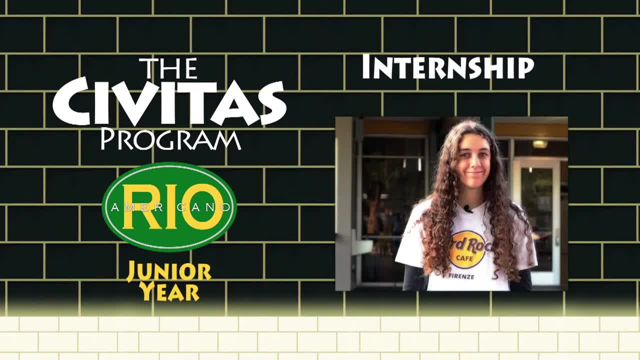 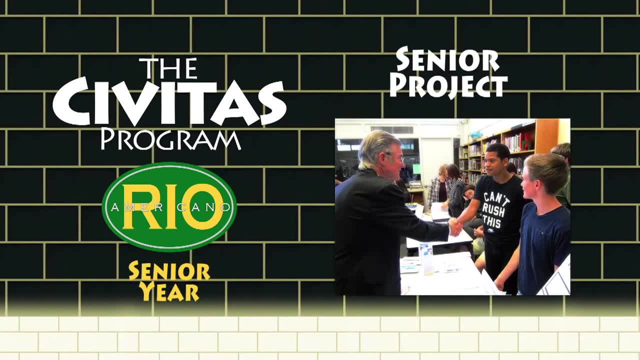 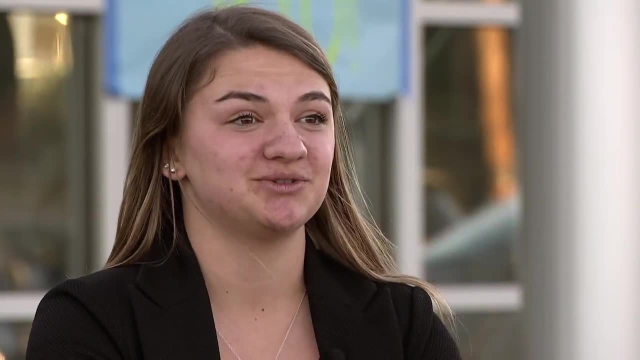 for youth organizations. Juniors take part in an internship, many of them working for state and local agencies, And students spend their final year on a culminating senior project. The Civitas program has been a presentation to a panel of community leaders. My senior project was a teen suicide awareness and. 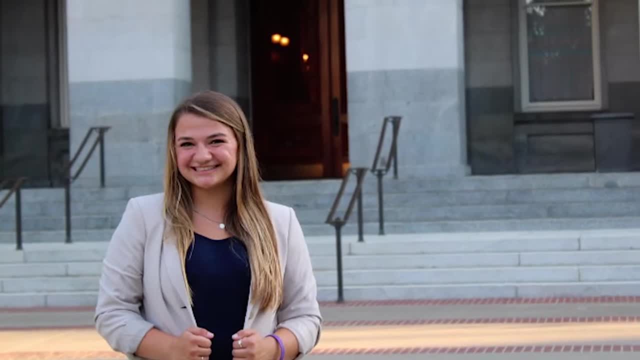 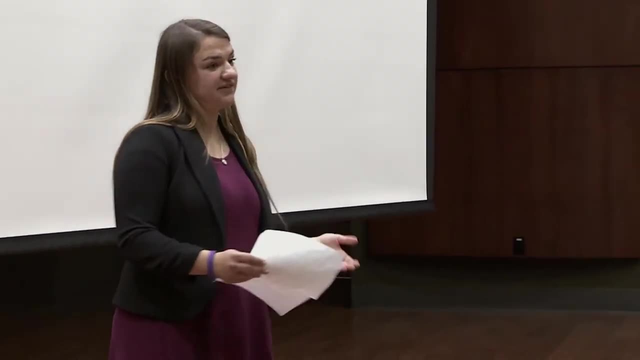 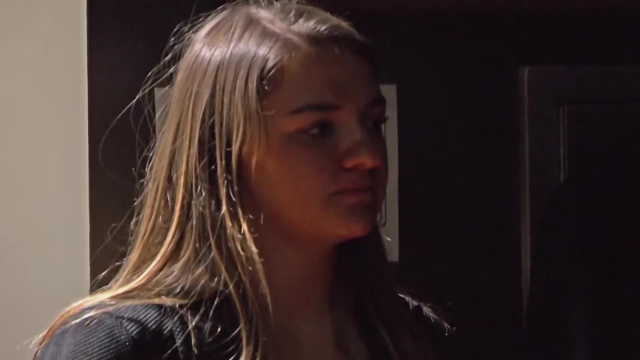 prevention campaign. Carolyn, who lost a friend to suicide, raised almost $1400 for the American Foundation for Suicide Prevention and she held a forum at school to educate other teens. She says the Civitas program has helped her define a path and practice the skills she'll need in the future. 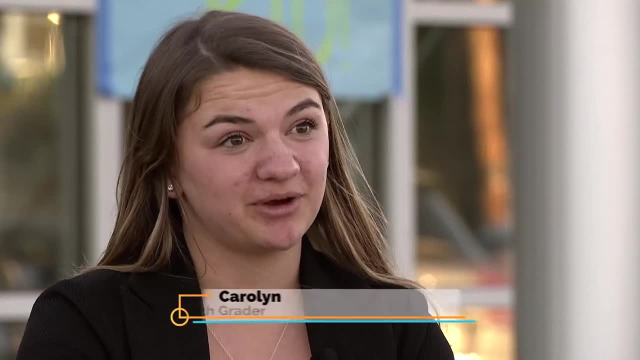 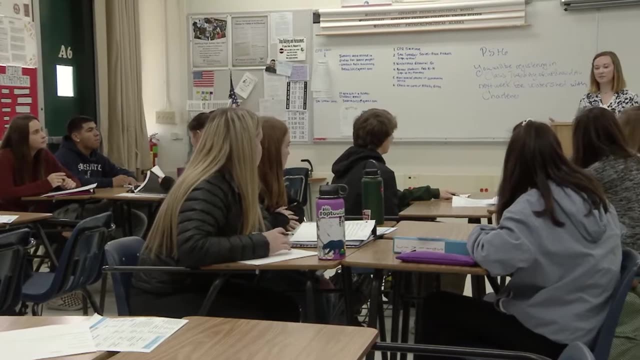 I think it'll help me not only with teamwork and leadership and collaboration, But on top of that it's kind of learning how systems work and learning how to get out there and make a difference In Civitas, like other high school civics programs, 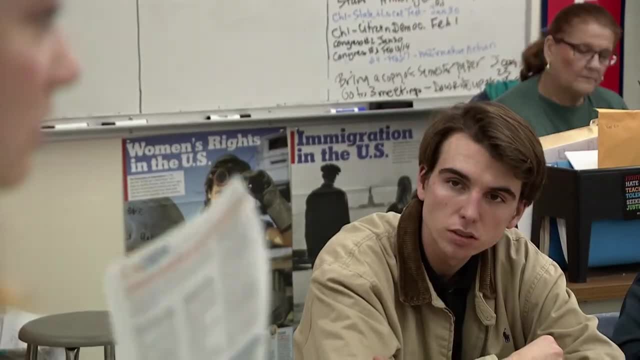 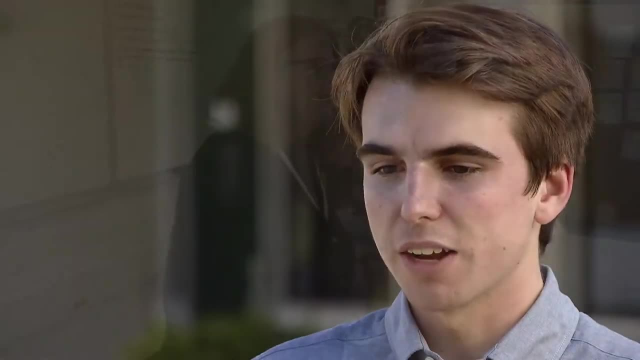 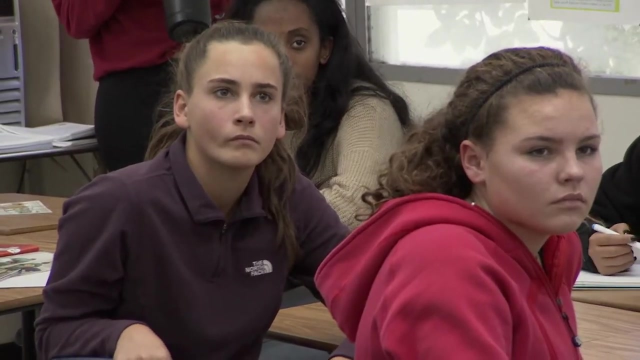 students are encouraged to disagree and taught to form opinions based on knowledge. So, Ricardo and Morgan, you guys are going to be pro and con. You're really not relying on textbooks or lectures. You're. the news is essentially your curriculum. Okay, so I'm going to give you until 10 after to read this. 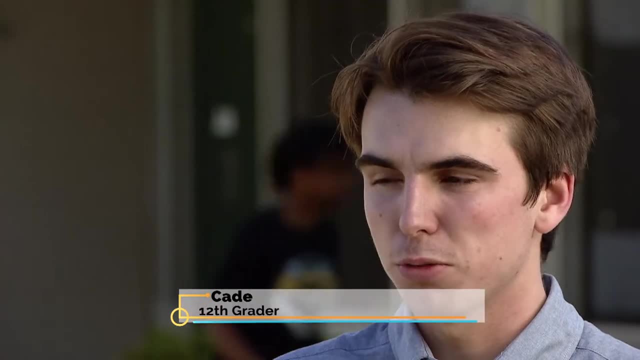 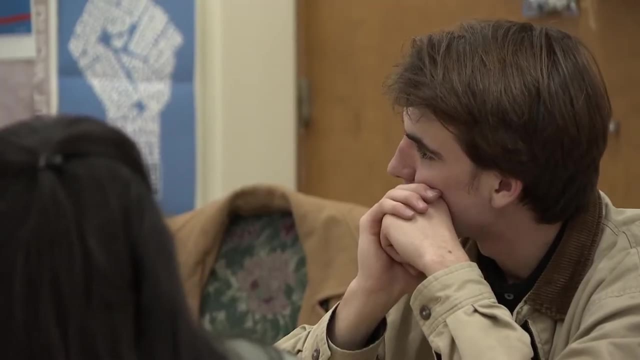 article and take notes on it. So there's only- You're talking about topics in class that most people are too afraid to bring up in an educational system, And so it teaches you how to listen effectively, how to communicate in the correct way. 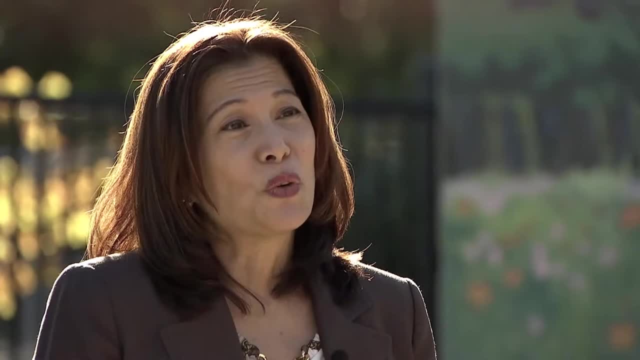 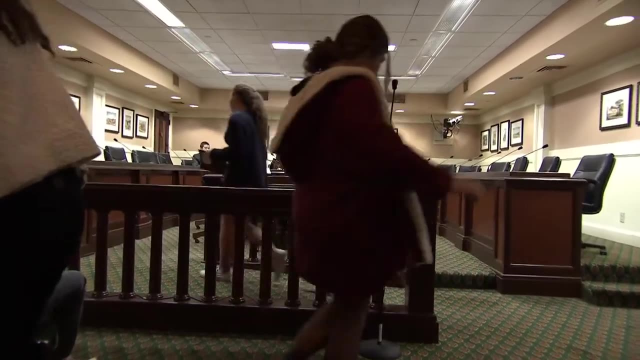 So there's just a lot of ways it shapes you to be a great person. It's never too early to start thinking about the future and your role in it and your voice in it. To be a leader, you need a number of skills, and these: 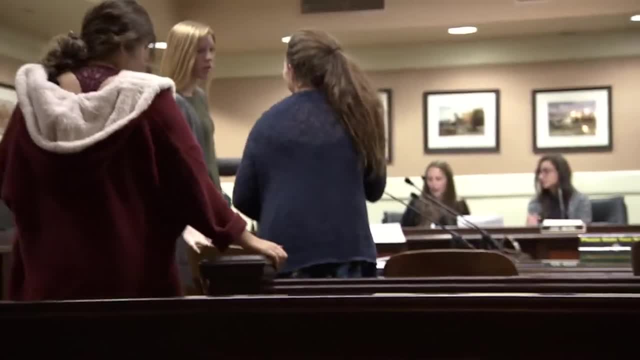 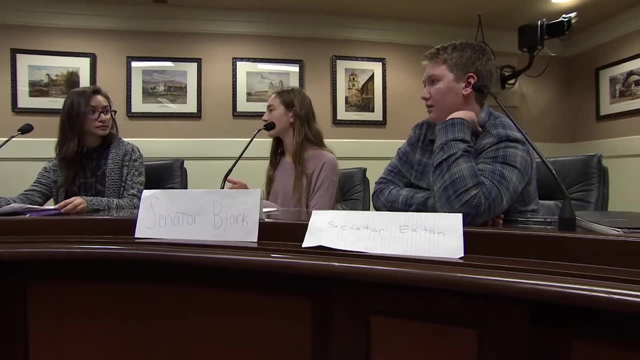 skills are best developed, I think, early on, so they can be honed. These students have thought about their futures perhaps more than most kids their age. With the internship, the community service, the focus on debate and the senior project, they've also begun to create a long-term academic and career. 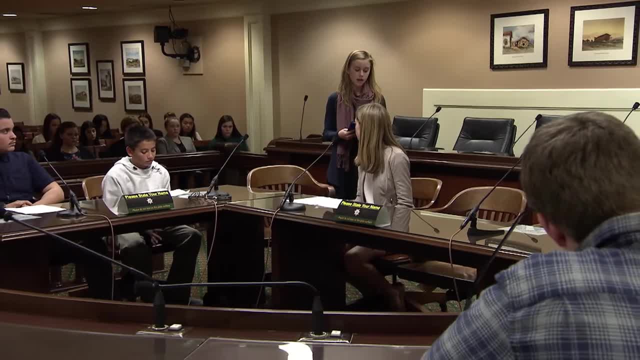 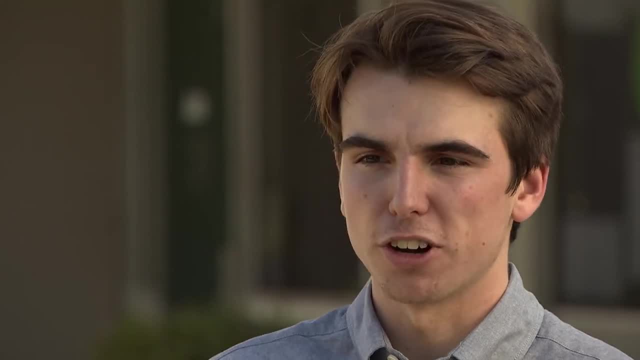 plan by building a strong college resume, perhaps without even realizing it. I probably wouldn't have done a 75-hour internship during the summer, or taken on an advocacy project or done 100 hours of community service if I wasn't required to by Civitas. 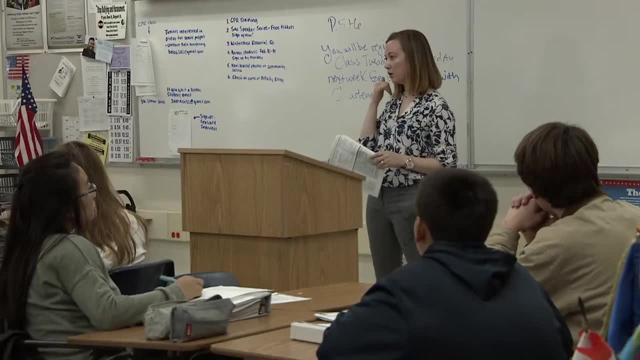 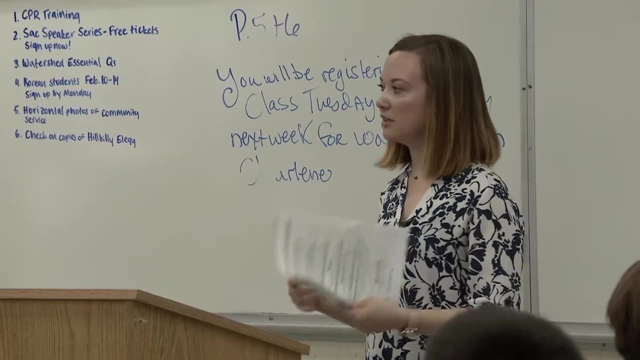 But because of that it really helped prepare me for college and, I think, just alone for college preparation and getting prepared to go out into the real world and like communicate. I think Civitas and civic education in general is like the best method for that. 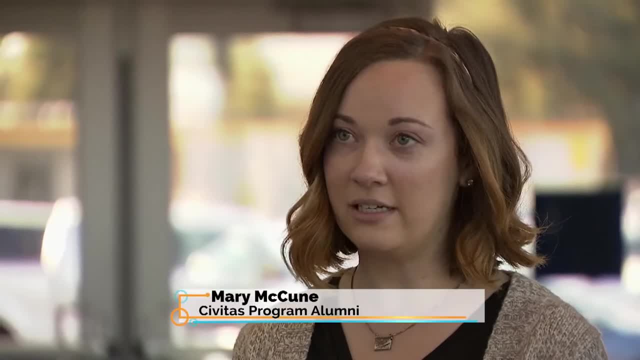 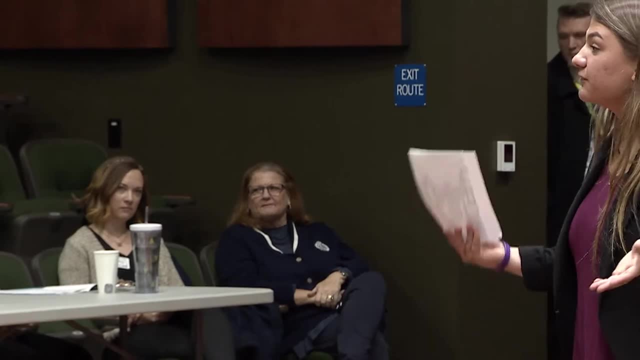 I think without these programs a lot of people would find entering politics and policy very intimidating. Mary McCune is a 2006 graduate of the Civitas program. She credits its enhanced curriculum for putting her on the path to law school and a career in public policy. 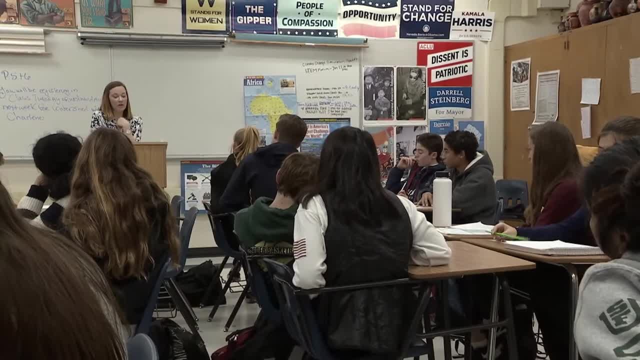 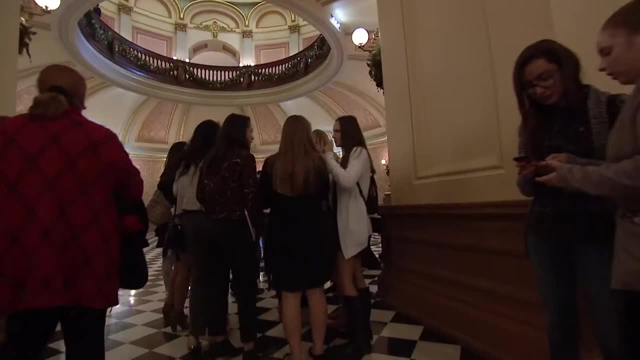 I had to go to city hall meetings. I had to go to county supervisor meetings. I was able to go and talk one-on-one with elected officials. It's that kind of experience, along with the chance to walk the halls of the state's capitol and sit just feet from California's top judge. 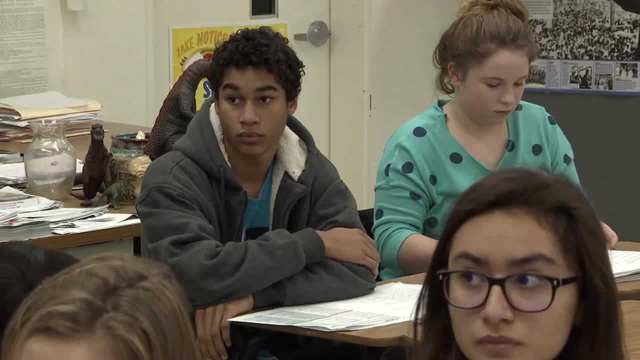 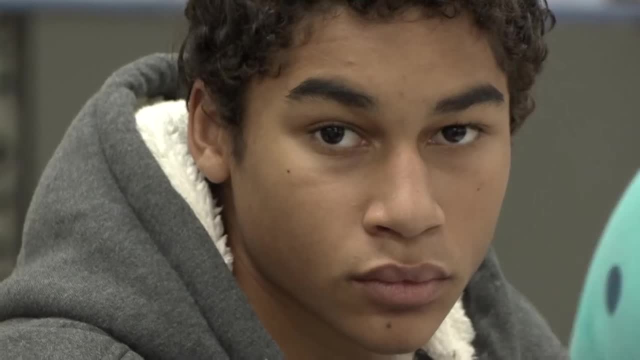 that gives students a peek into the future and a reason to look forward to three more years of high school, years that these teens all agree are helping to shape them. I'm really excited for the next three years. Honestly, I'm still trying to figure out. 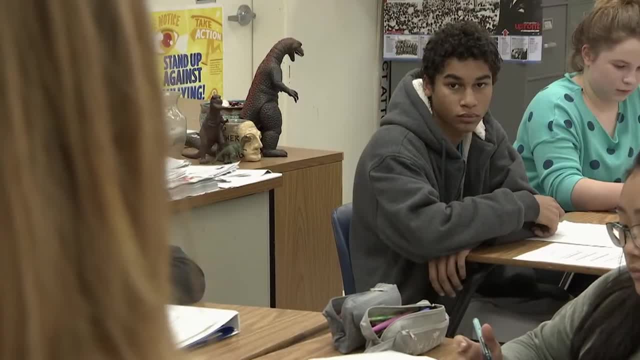 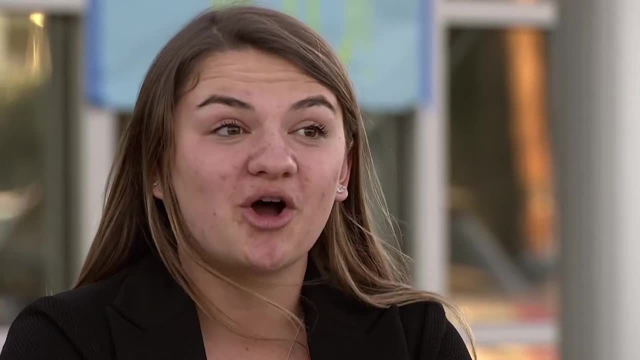 okay, Aiden, your senior project, your junior internship, it'll be fun. I look around and I see the brightest faces and the brightest minds and the brightest ideas, and whether or not we agree on certain things, each and every one of them know how to compromise and 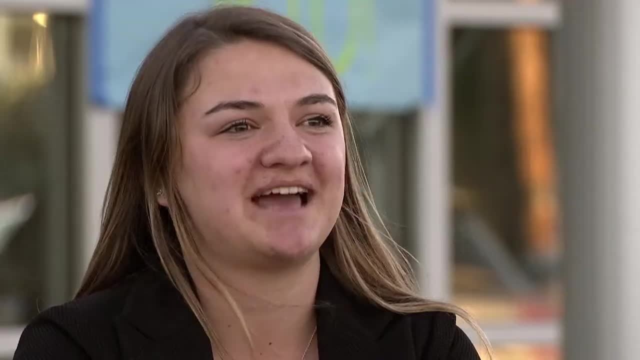 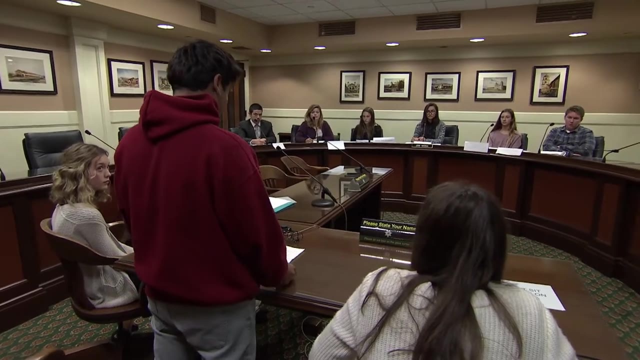 that is exactly what we need for the future generations, especially in politics, and advocacy is compromise. So now they're kids, they're probably able to discuss politics and government with adults on a really easy basis. and now they're going to be adults and they're going to be really well informed adults. 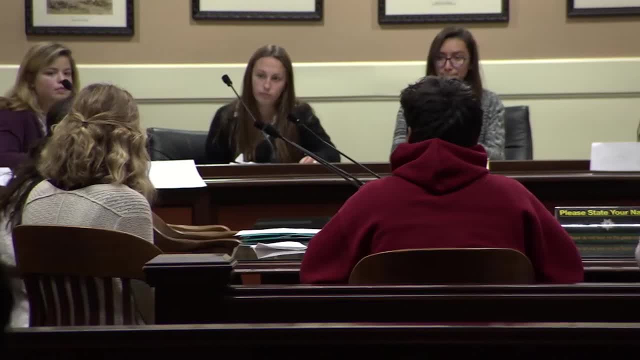 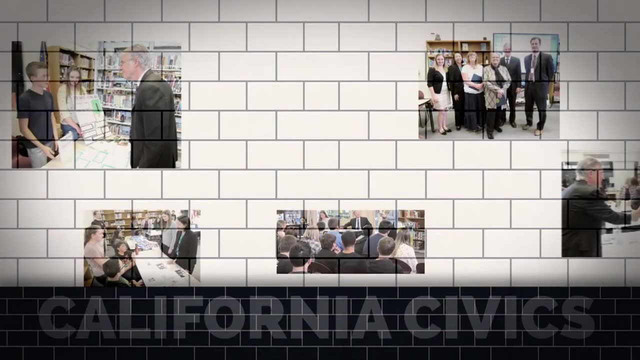 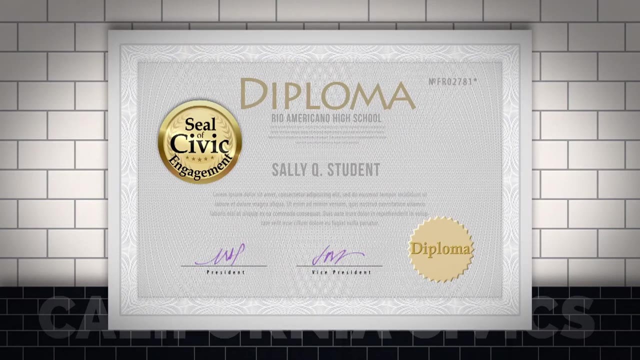 Adults who will also be well equipped to take the helm as our state's next generation of leaders. Students completing programs like Civitas will soon receive a California seal of civic engagement on their high school diplomas. It's the result of new legislation expected to take. 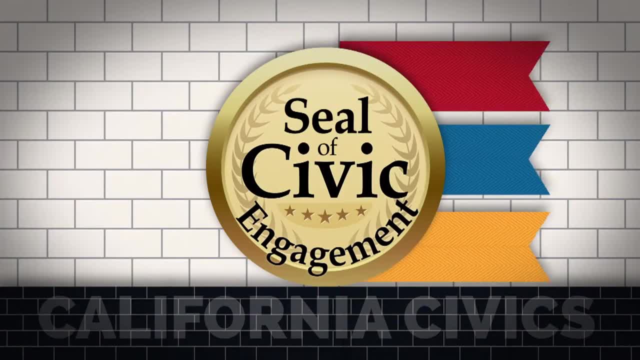 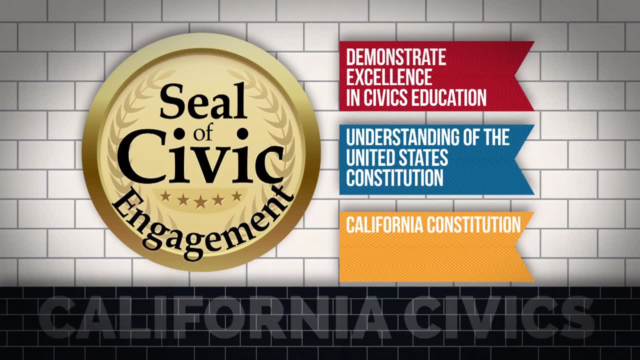 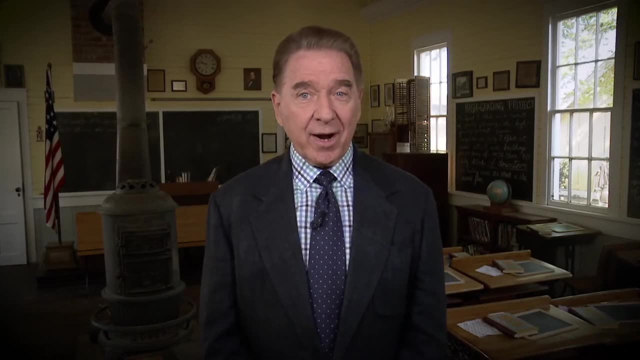 effect in 2021.. The seal will be awarded to students who have demonstrated excellence in civics education, with an understanding of the US Constitution, the California Constitution and our democratic system of government. Let's journey next to a school in San Diego where 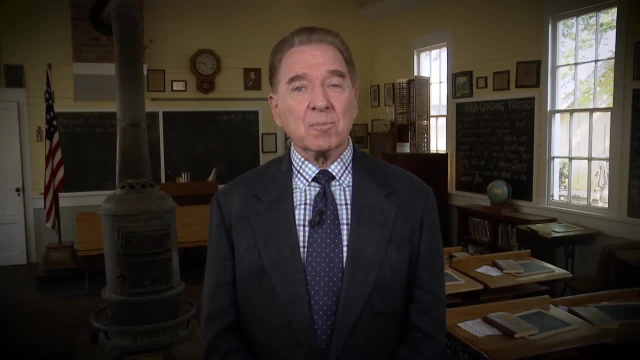 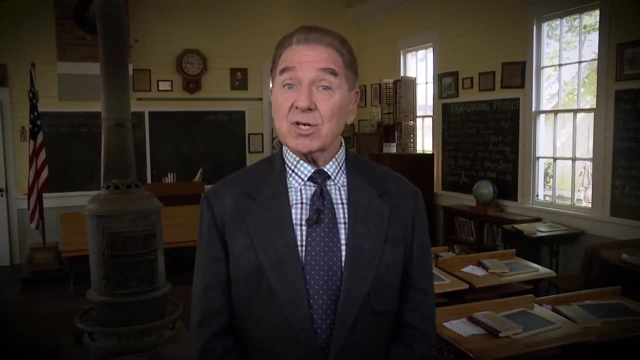 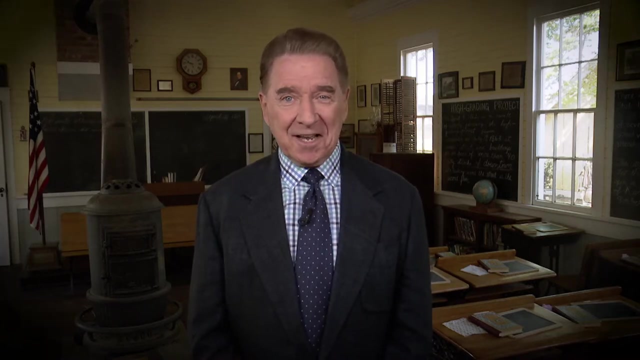 dozens of students participate in a military themed program called Junior ROTC. The goal of the program is not to enlist students in the military. instead, it's designed to help them develop the maturity, discipline and leadership skills they'll need to succeed in life. 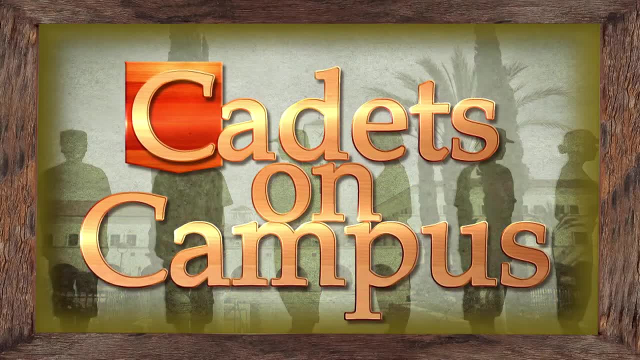 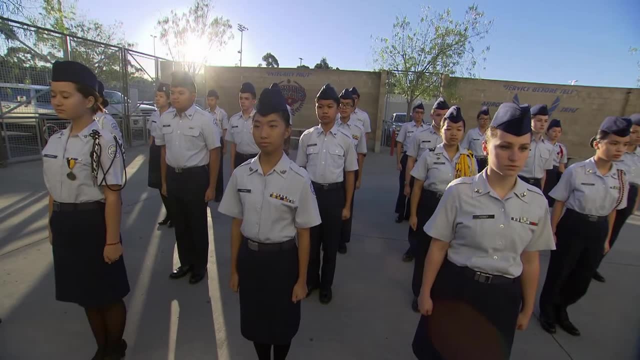 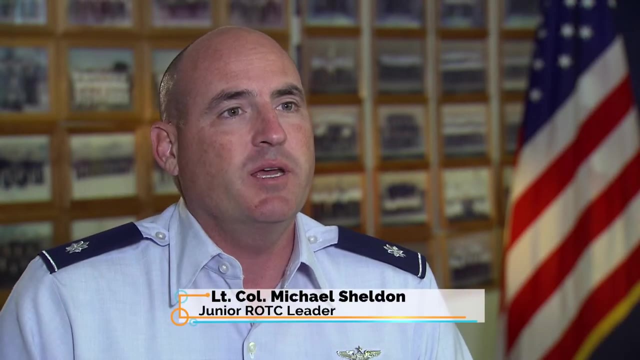 4,, 3,, 2, 1.. Up on the flight sit hut, The idea we're trying to do is build citizens for the United States, build a sense of responsibility, patriotism and hopefully overall, some life skills that they can use later on. 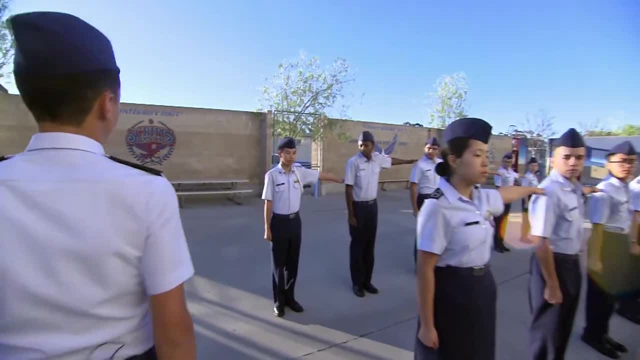 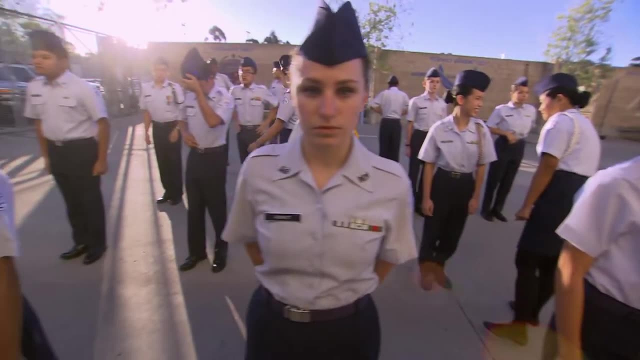 Lieutenant Colonel Michael Sheldon admits that a military uniform inspection might not be what you're used to seeing at a California public high school, But this Monday morning activity is a regular feature of the US Air Force Junior ROTC program at Scripps Ranch High School in the 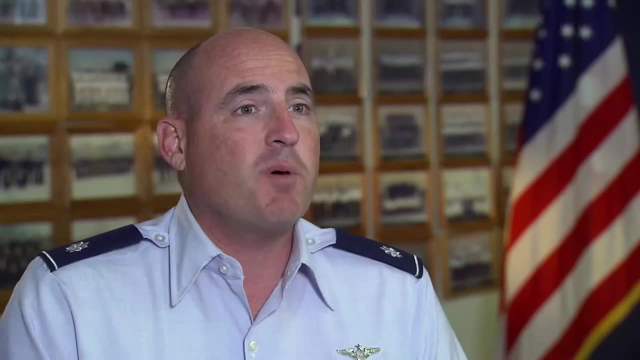 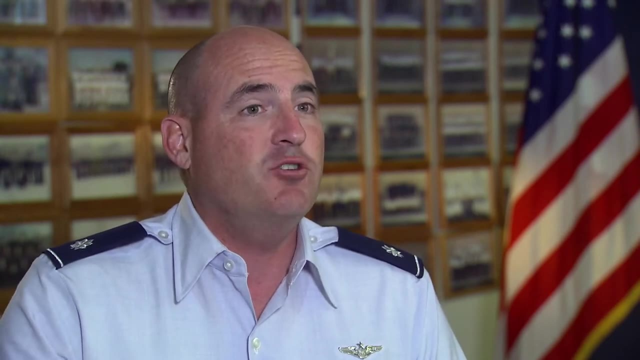 San Diego Unified School District. The students wear their uniform on Monday Just to make sure they maintain their uniforms, get that attention to detail. they have an inspection and that's led by a junior who's a flight commander And they'll go out. look at their uniforms. 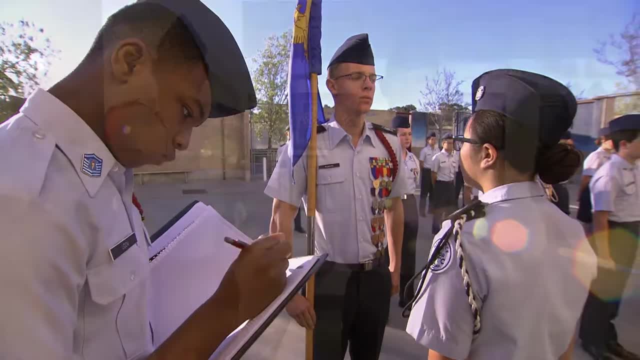 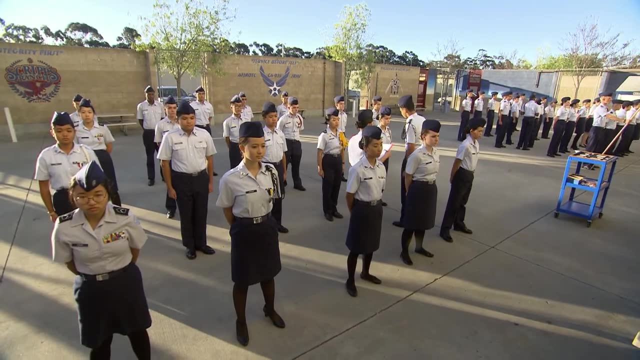 see if it's in proper condition. it's clean, they've shaved, they've shined their shoes. Colonel Sheldon and Master Sergeant Ferdinand Toledo oversee the 173 young men and women who've chosen to join the ROTC unit as part of a high school elective. 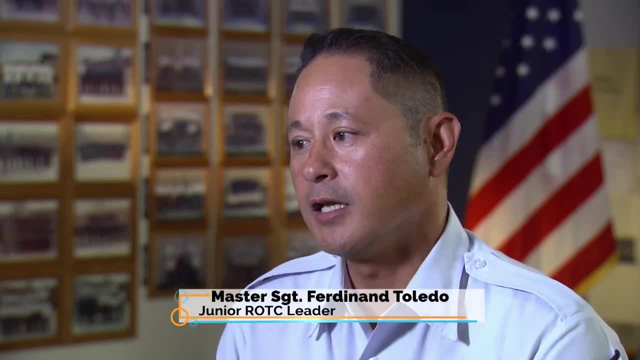 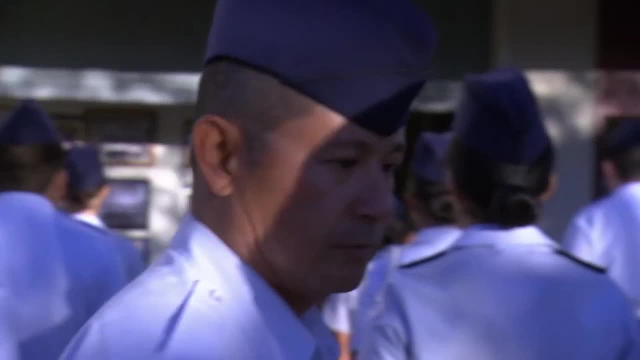 In the San Diego Unified School District there are 17 high schools, and out of the 17 high schools 13 are military. We have 14 have Junior ROTC units, And not just Air Force but across all services. The Junior ROTC program began here in 1993.. 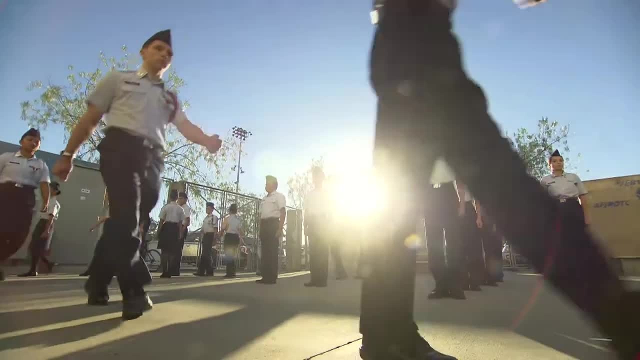 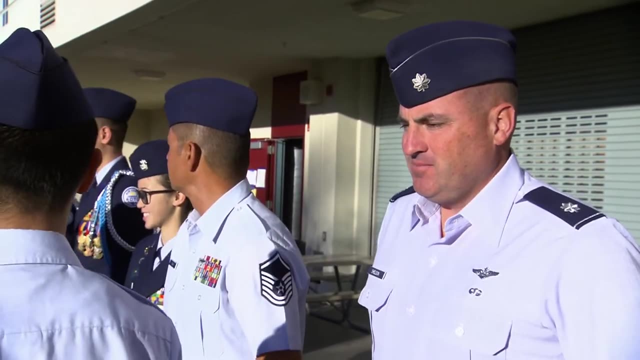 Mondays require the students called cadets to wear their school provided uniforms for inspections and award ceremonies. The uniforms are a new experience for most. I don't have any cadets that were excited to wear it the first time. It's something that makes you stand out for sure. 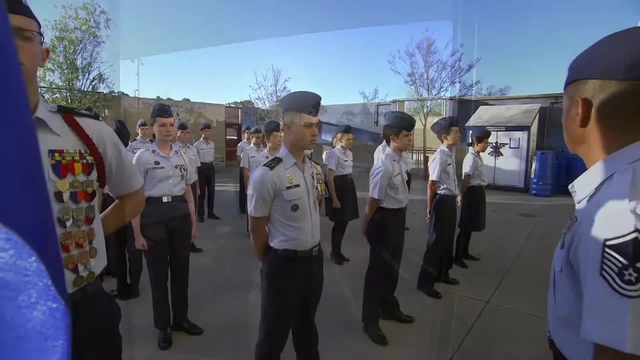 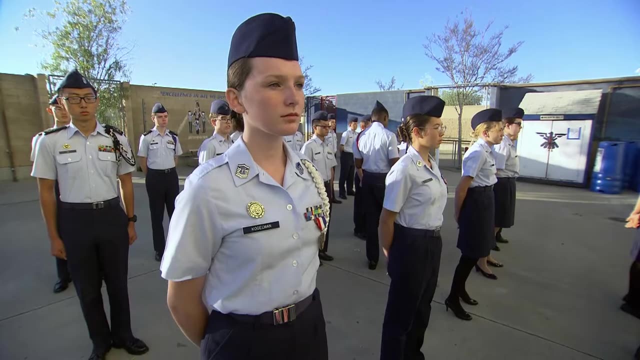 But I really think it just comes down to wearing it proudly and to embrace being part of the program. It's something I enjoy. I always love Mondays because, firstly, I don't have to worry about picking out something to wear And, secondly, we're all wearing the same thing. 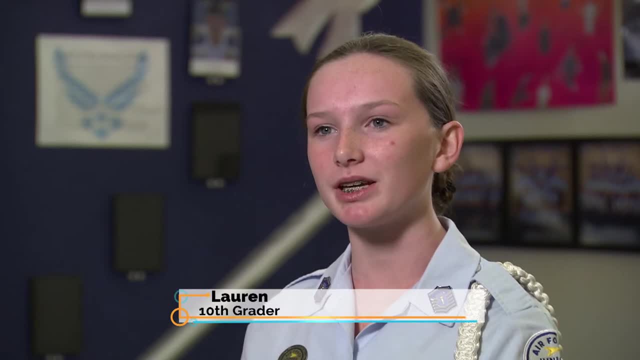 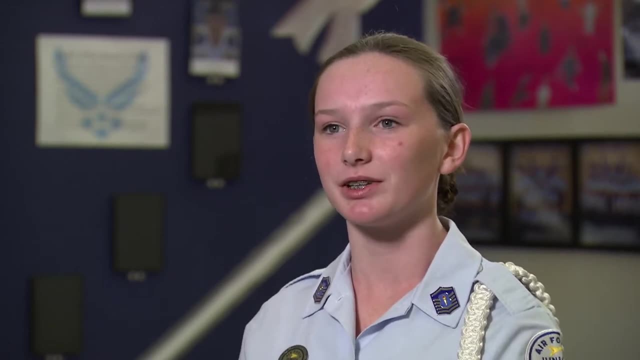 It shows unity And personally I'm very proud to wear this uniform because it shows I'm a part of this program and it also shows that, in a way, I'm linked to the Air Force, And that is just an amazing privilege. I pledge allegiance to the flag of the United States of America. 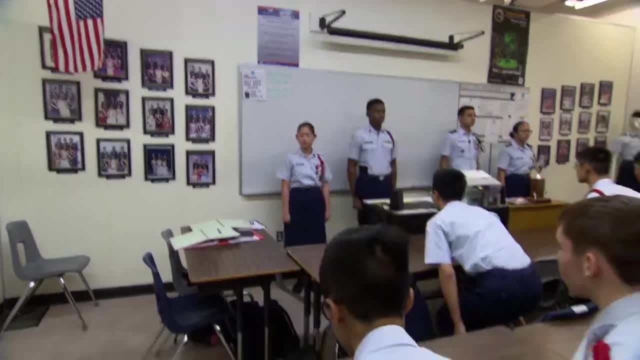 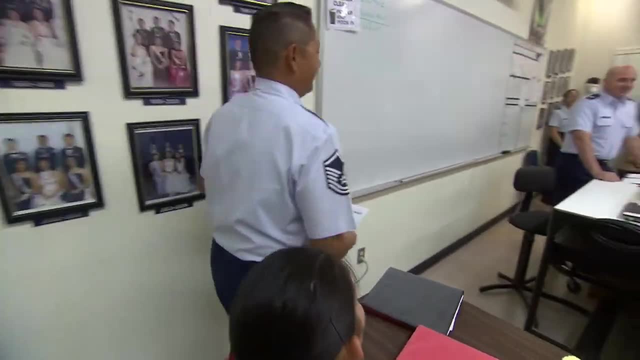 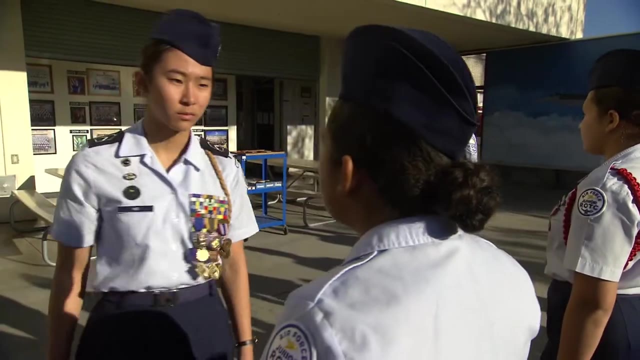 In words, face cease. Happy Monday. Are you guys awake already? Are you sure Let's go ahead and turn to page 170.. 170. The ROTC program demands not only the Monday inspections but regular class work and physical education requirements. 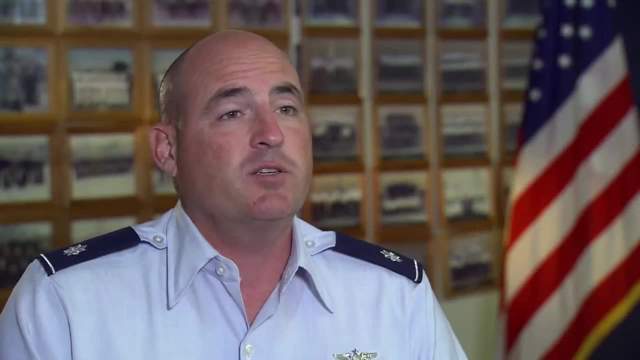 It's every day of the week: Monday we do the inspections. Tuesday we have academics. Wednesday, Thursday: physical fitness. Friday: academic again. So we have a set week And every day And every five periods we have students here. 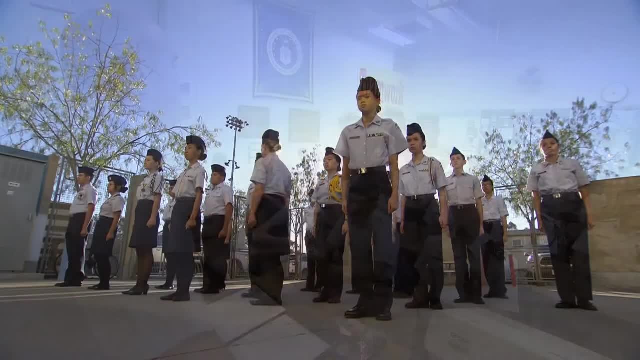 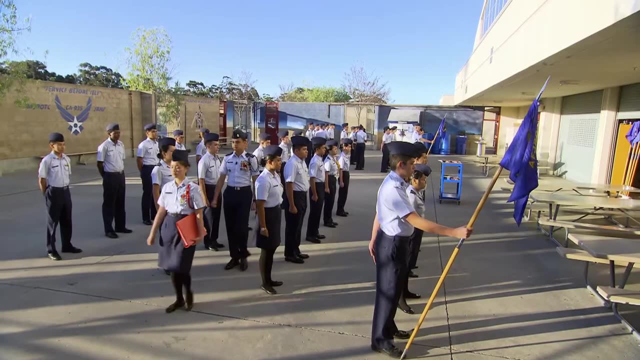 The focus here is not only on academic requirements, but on using a military training approach to help cadets move up the chain of command and take on greater leadership roles. For Lauren, it was a way to no longer be self-conscious. I just knew that something was going to happen. 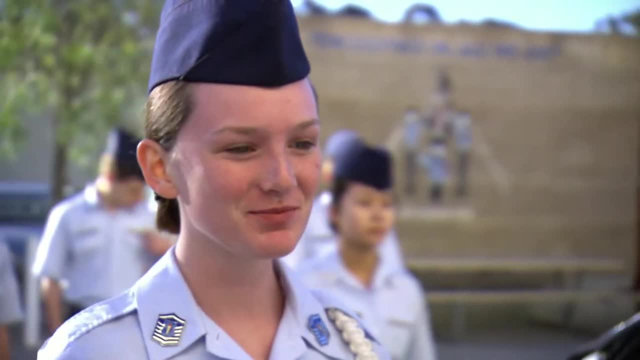 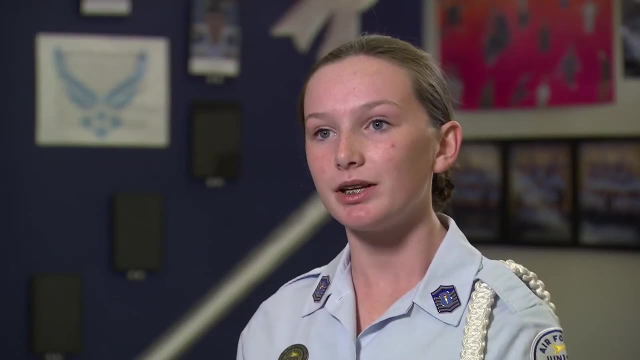 There was going to be a change. I knew that here I would have the opportunity to succeed just by being myself, And that's something I've not really had before, And this would be the best place for a fresh start. It's a solid community where I can make friends and have a 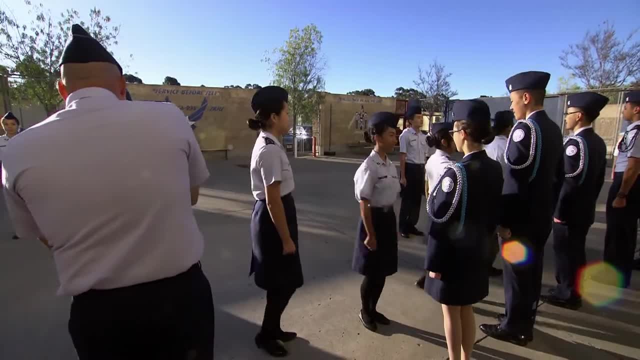 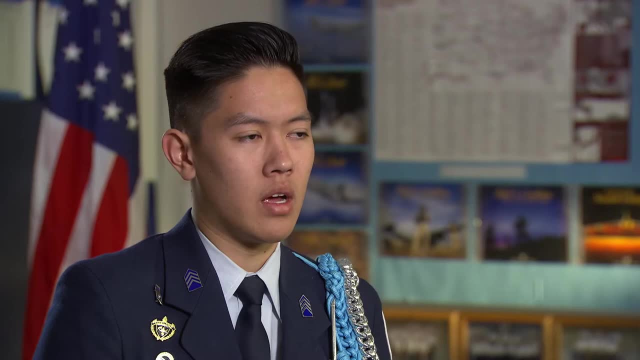 place where I can belong in the school. I think the best benefit was leadership experience. in middle school I was a very shy kid So I didn't really have many friends. I was in a small group But moving to high school I needed to branch out more and 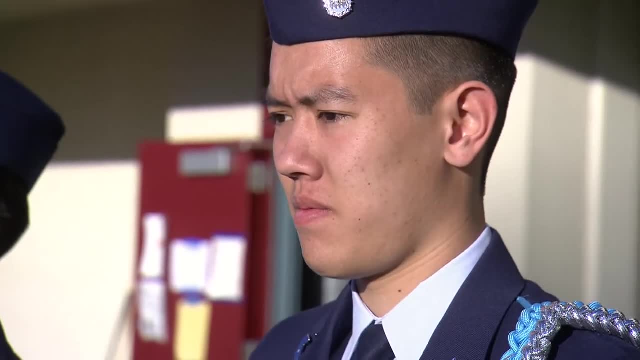 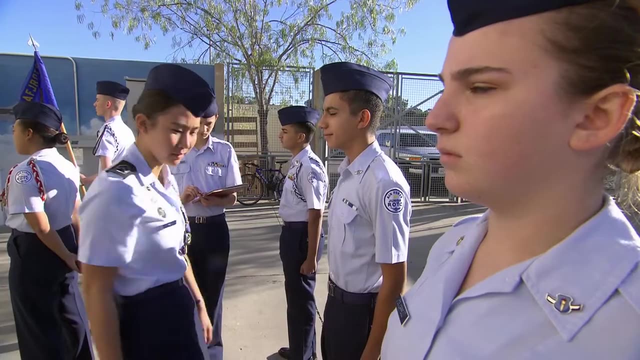 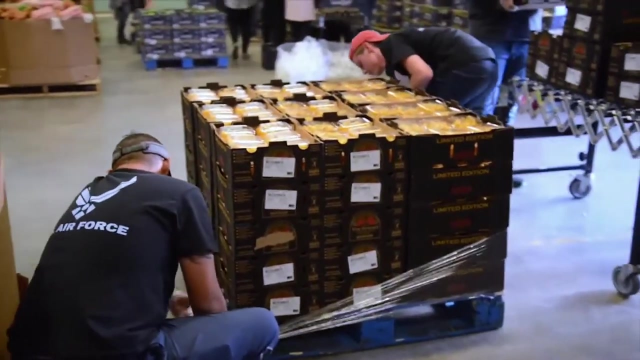 find myself, And this program definitely helped me do that. The goal of Junior ROTC is to prepare these young people to be good leaders, to be confident, to be accountable for their actions, And we teach leadership, education and life skills. Community service is also part of the ROTC program. 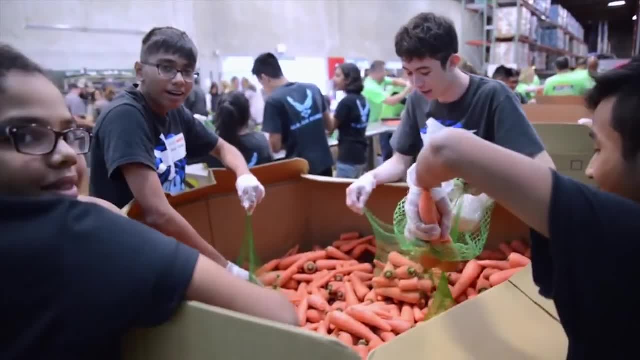 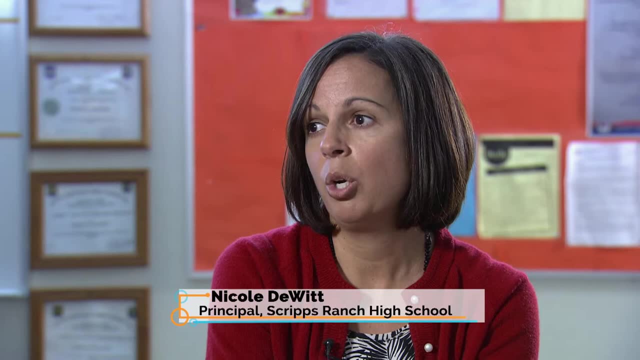 Outreach to food banks, school tutoring programs and presentations. It really takes leaders to step up and do that, And I think a lot of the students that participate in the program really find those leadership skills and hone those leadership skills while they're here, And so it's definitely something that I hope they take away from. 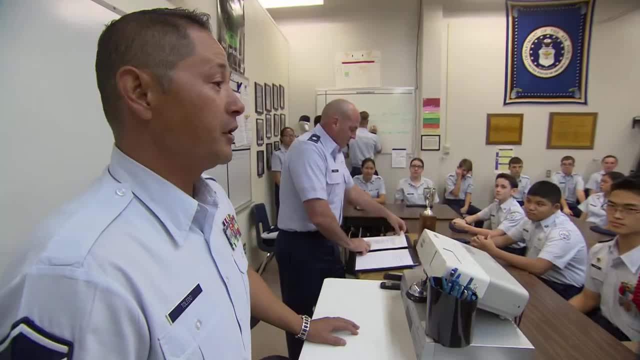 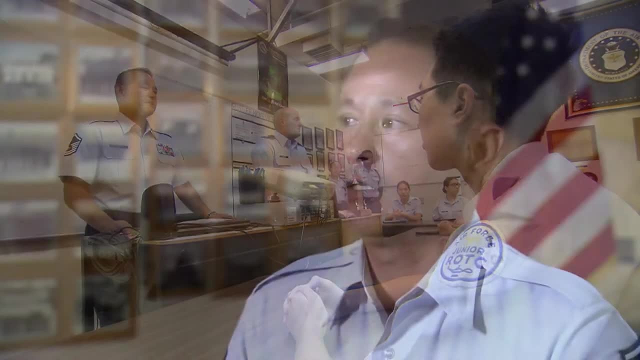 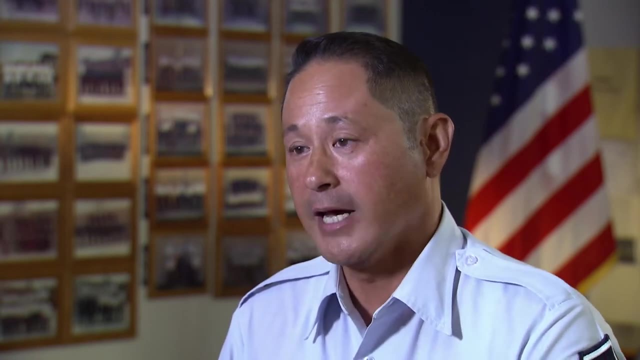 it. Many might think the program is focused on encouraging students to consider a career in the military, But the school is quick to point out that's not the case. Statistics in terms of the Air Force Junior ROTC unit units across the country: less than 2% collectively actually join the. 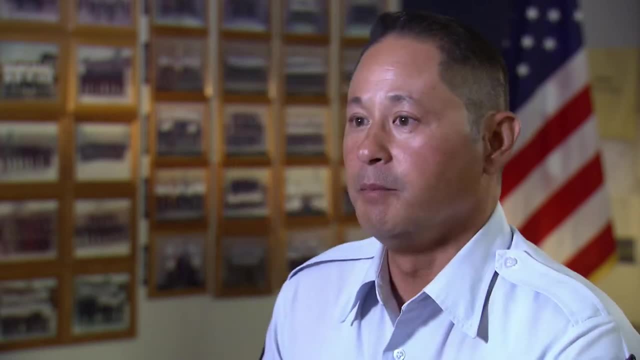 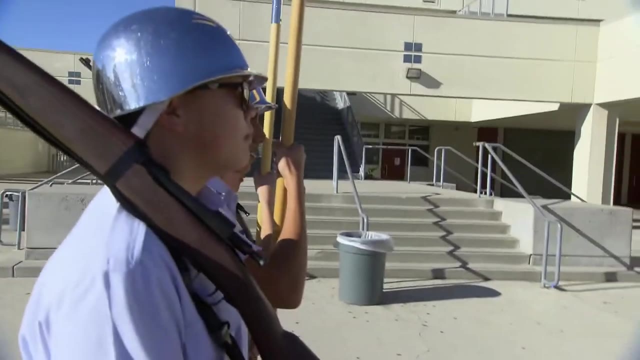 military or some sort of category of the military? Left, left, right, left turn. Many of the cadets also choose to take part in the unit's extracurricular activities. Nisa is a freshman who liked what she saw in the color guard. 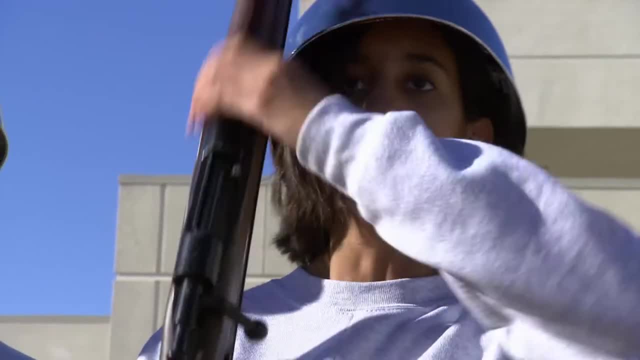 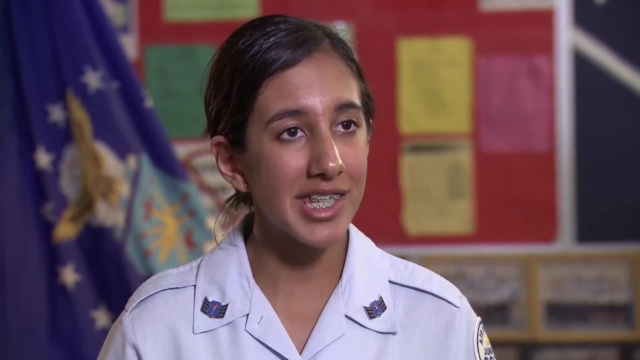 unit. You have to work with the team together, You have to be entirely in sync the entire time And you have to know how to hold your equipment and just work together as a team to make your performance as sharp and as nice looking as possible. 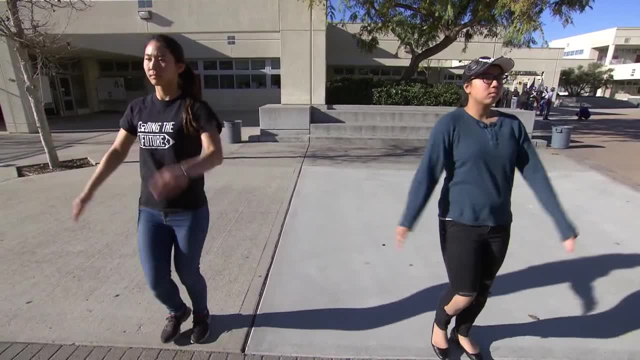 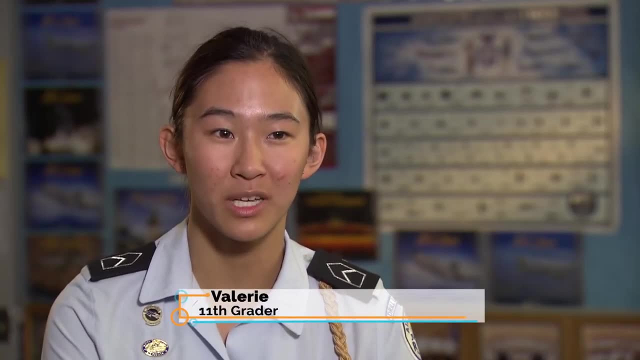 We have four drill teams. It's the unarmed team, the armed team, saber team and color guard team. I'm on the unarmed team, So that one. we don't use any weapons, It's just making rhythms and beats with our hands and feet. 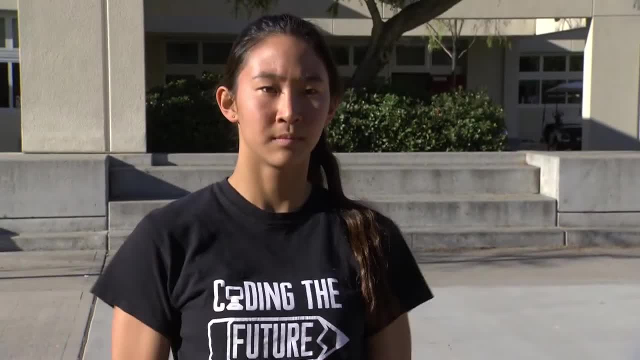 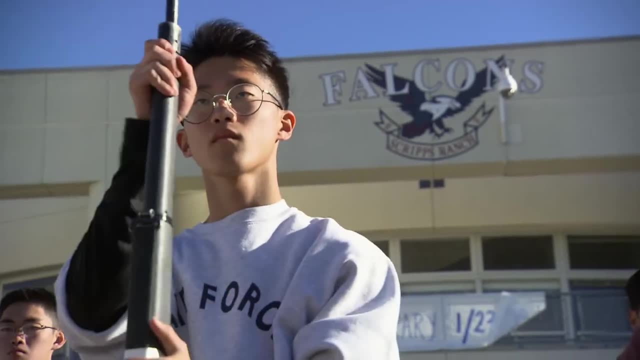 We all compete at four times, So we have up to five competitions each year. Ready move. Our rifles are black and we have a red and white tape design on them, So when we throw the rifles people are like: wow. The unit's award winning drill teams are not the only. 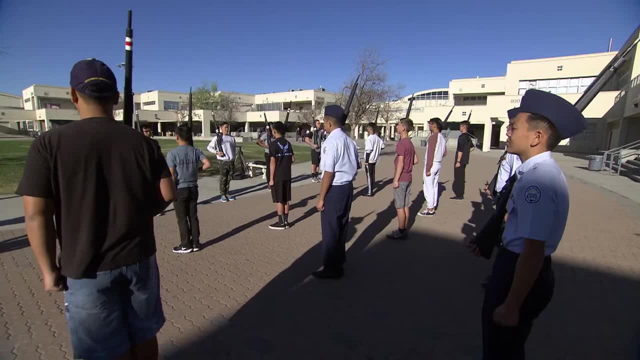 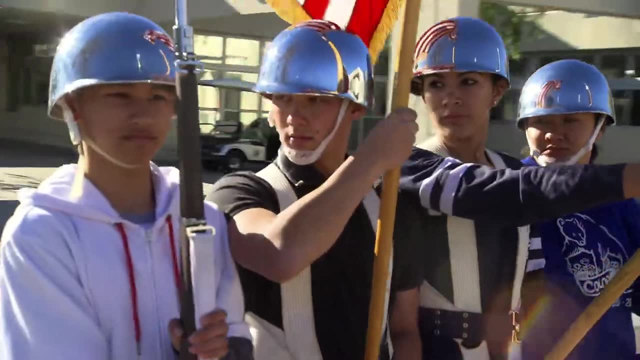 extracurricular activities for the program. Student academic and computer teams have taken top honors in national competitions, Like the American Eagle. The American Eagle is a national sport. It's a great sport. It's a great sport. It's a great sport. 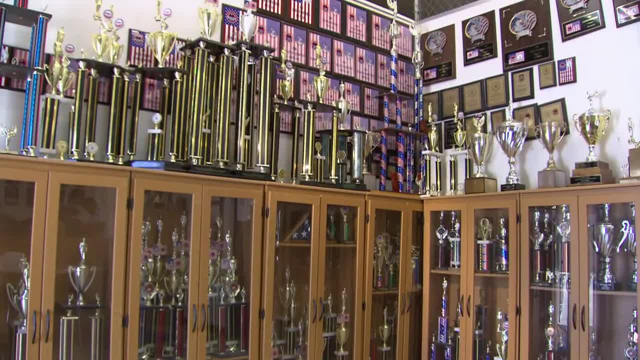 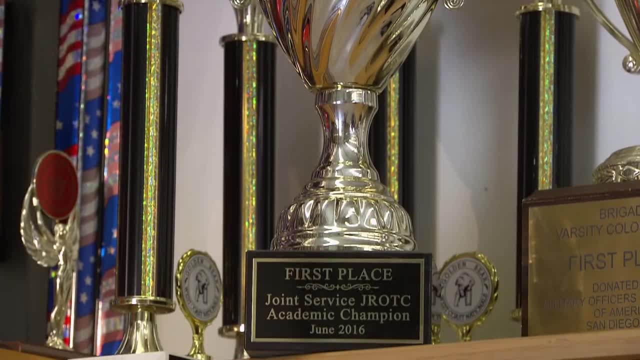 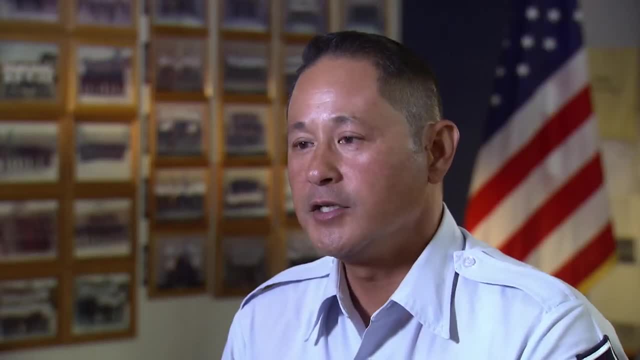 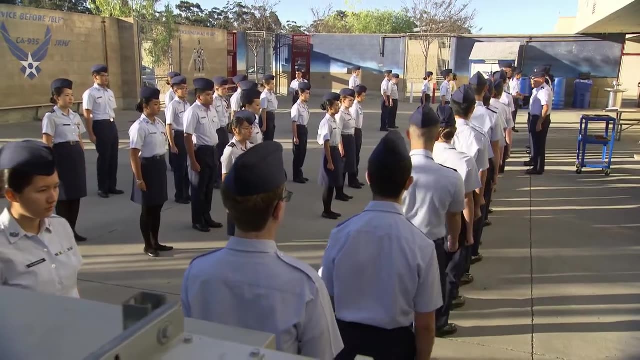 will serve them well as they go through life. They come back year after year and they tell me just how much the Junior T-Z Program has helped them with their confidence, with their ability to succeed, with their drive and determination on what they want to do. 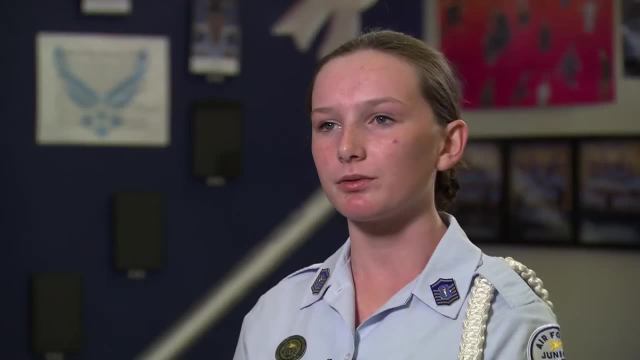 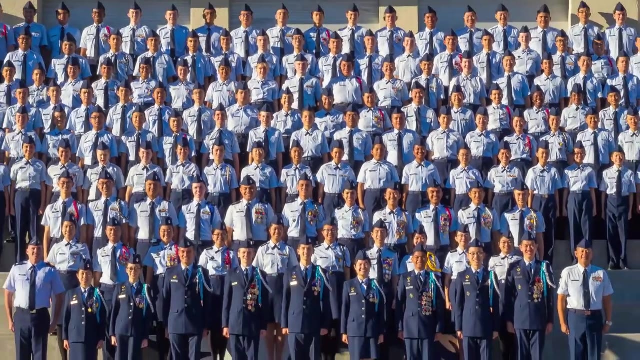 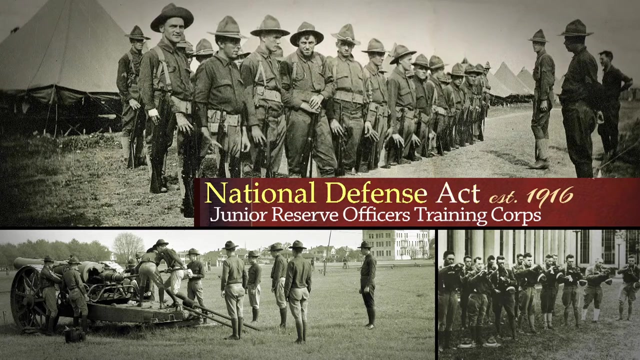 Congratulations Being able to meet so many wonderful people from so many backgrounds and being able to learn something from each and every one of them, and something that makes high school a. The Junior Reserve Officers Training Corps was established by the National Defense Act of 1916 as the US prepared to enter World War I. 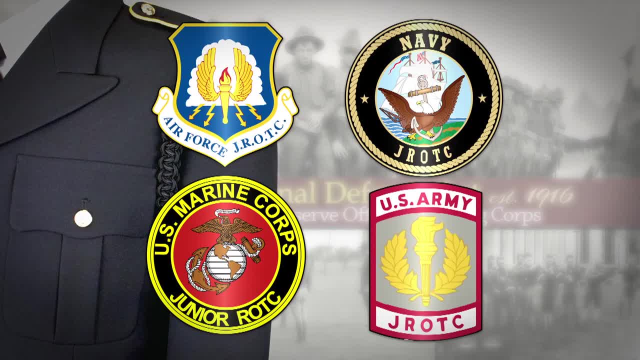 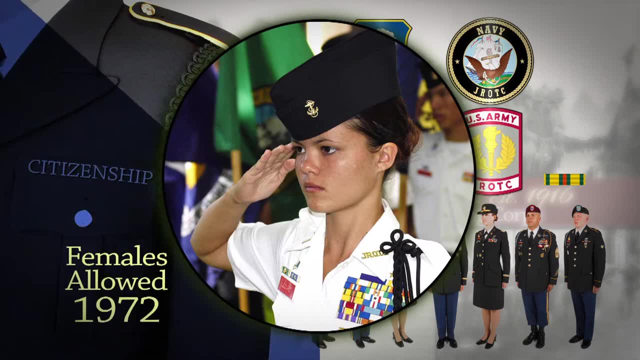 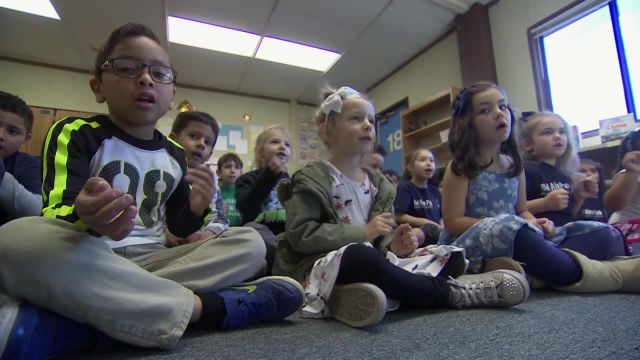 The program has changed greatly over the last century. Originally designed to prepare teams for military service, its focus today is on citizenship. Females were allowed to join in 1972. They now make up 40% of cadets. Still ahead on Inside California Education. discover how the International Baccalaureate Program 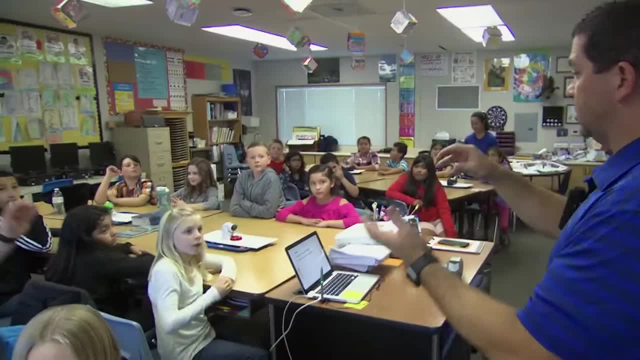 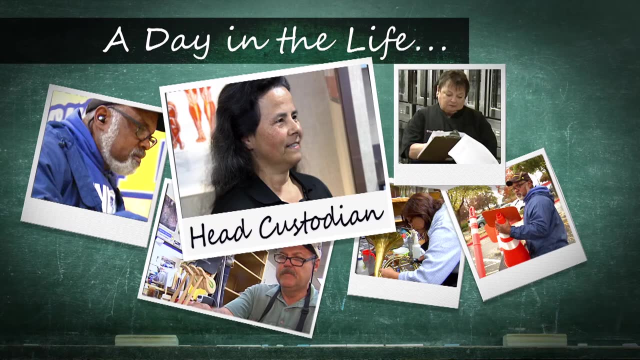 is teaching kids to think independently, ask questions and see both sides of complex issues. But first let's spend a day in the life of a school custodian. What I do is just about everything. Just about everything. If it needs to be cleaned, I clean it. 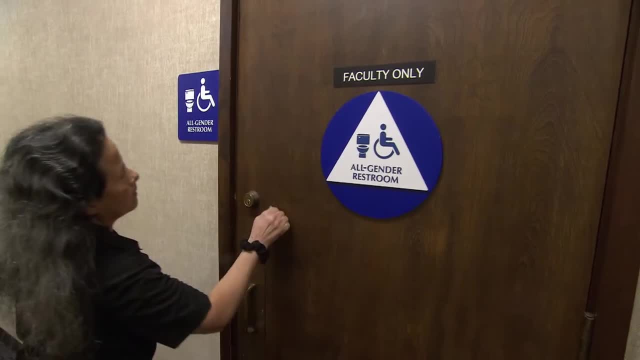 If it needs to be fixed, I see if I can fix it. What I do is just about everything, Just about everything Custodian. We're the eyes and the ears We're constantly looking around. Is that dirty? Is that safe? 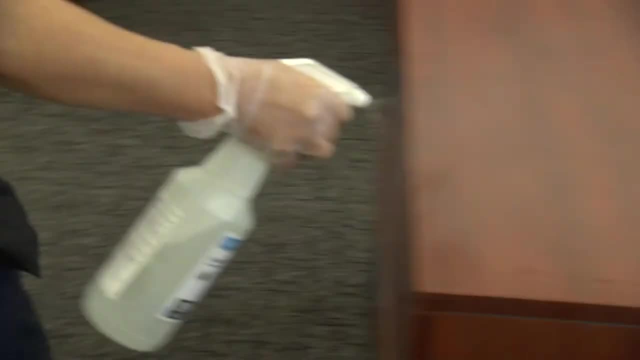 Is somebody going to trip on that? Let's take care of that now. My name is Mary Montes. I am the maintenance custodian, the night custodian, for Placer County Office of Education, the CTE building which is the Career Technical Education. 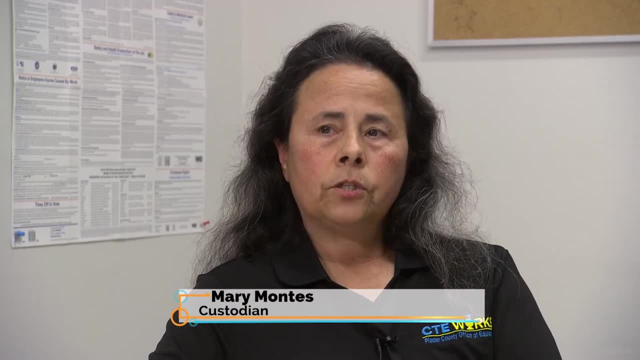 Miss Ellie, are you here? Every day when I come in, I check in with all the teachers, see if they have any needs, see if they have any questions. I'm here to help. I'm here to help. I'm here to help. 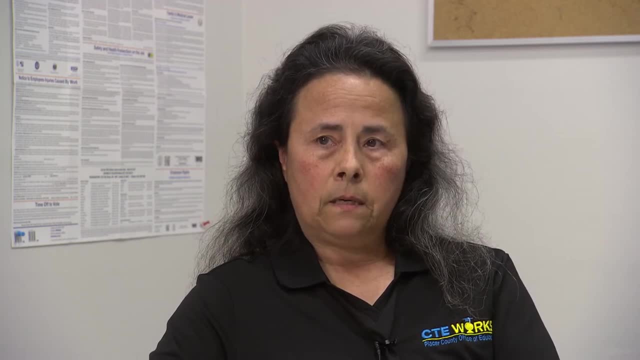 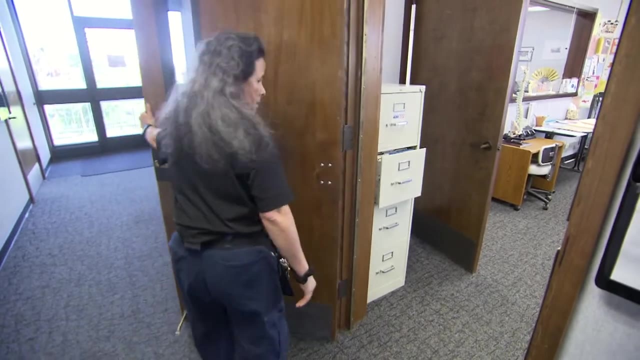 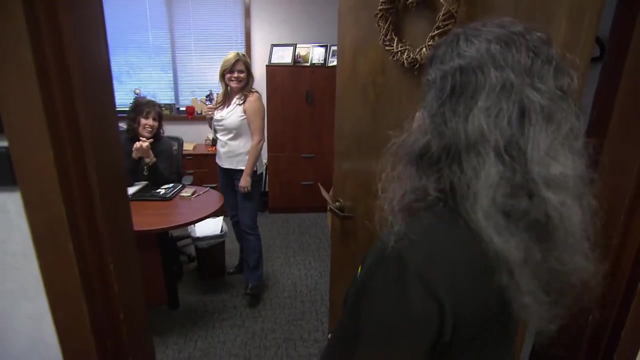 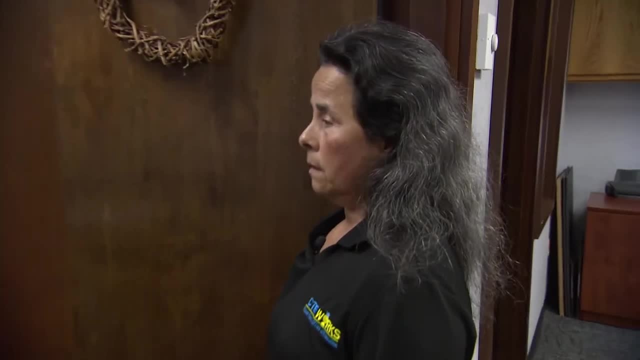 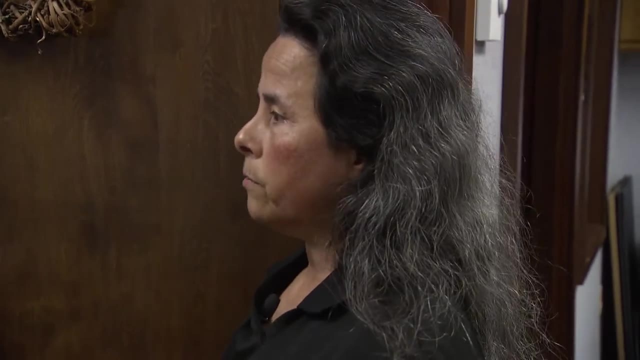 Do they have a special project coming up? Things are good. Okay, Remember, next week we have our visitor on, That's right. Assemblyman Kevin Keighley is coming to do a walk through, and I want the place to look beautiful. 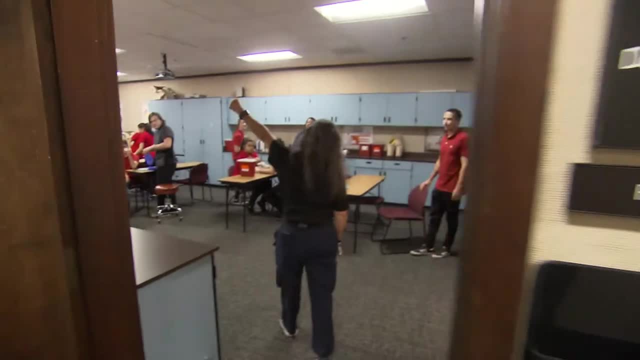 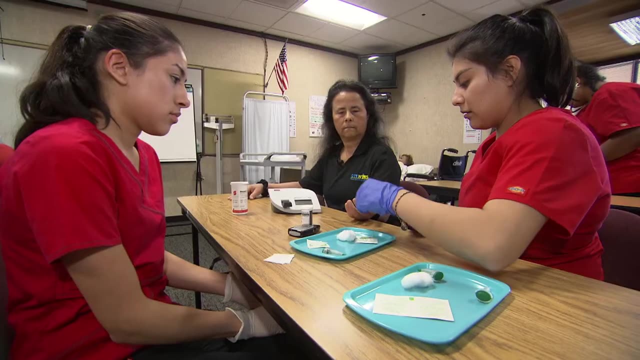 This is a career school. this is where the kids learn a career. You need a volunteer, Yeah, So if someone can do a blood sugar on Mary, I said I have an arm, you need one. So they go ahead and they do it. 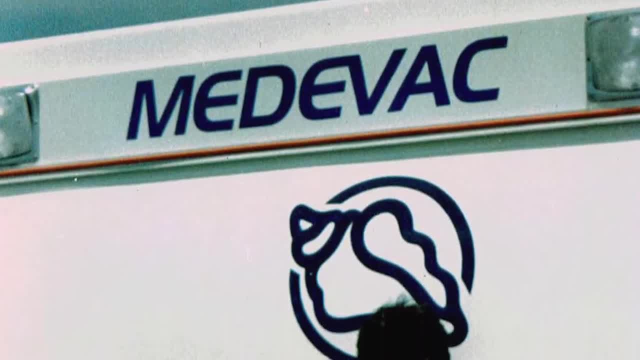 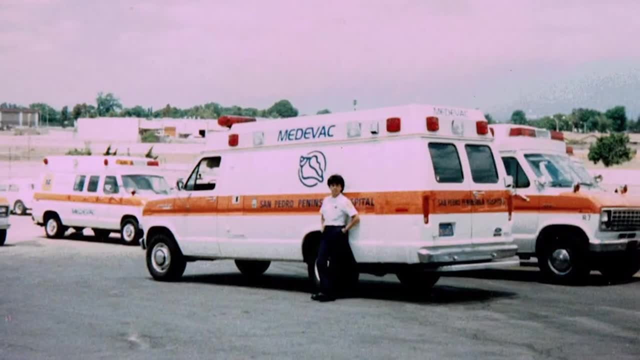 Thank you very much. You did a great job, both of you. I was an EMT for a number of years. I was with Medivac Ambulance. I learned how to be a medical assistant. I learned in a career center like this. 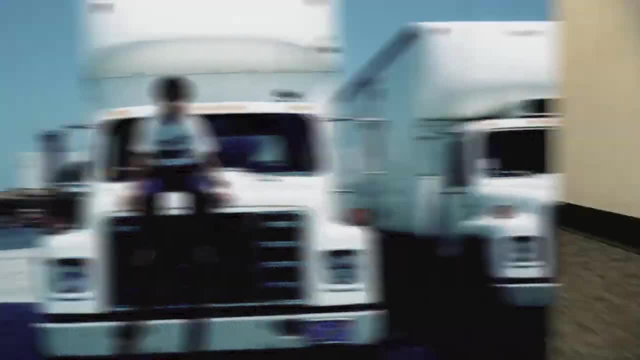 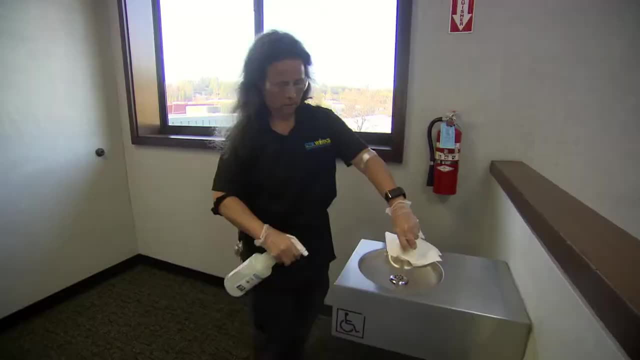 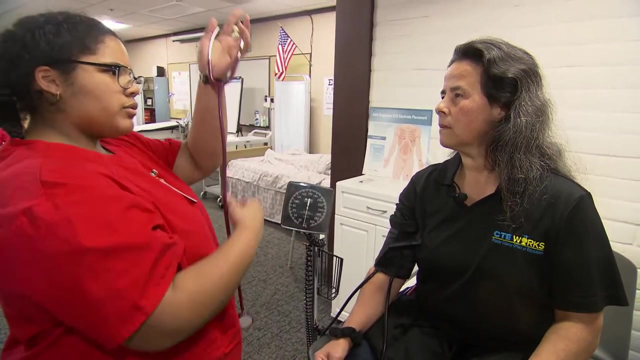 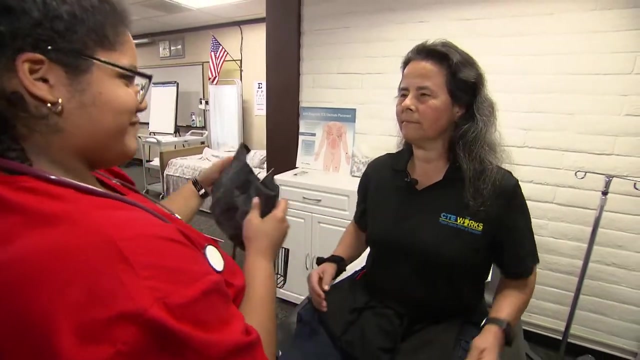 I've been a carpenter, I have been a truck driver. I like interaction, I like talking to the kids, I like talking to the people And I also like being able to just do my job and just be left alone. So I get the best of all the worlds. 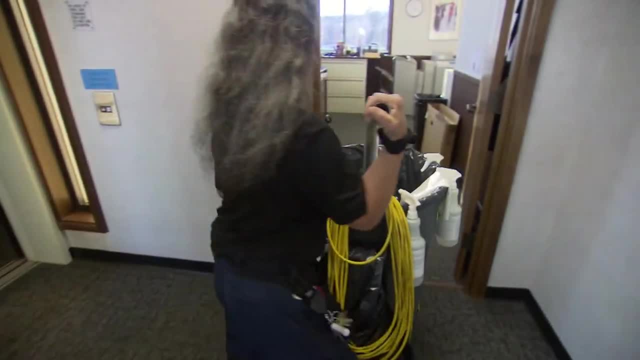 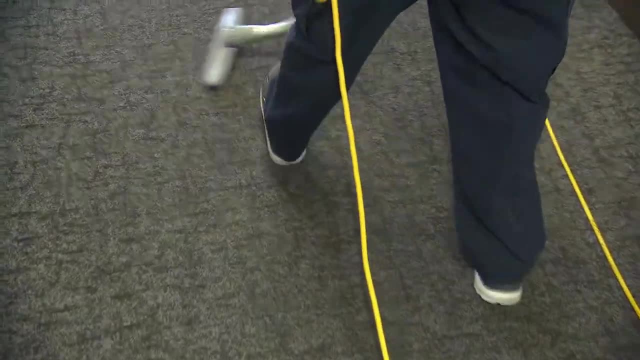 Have a good evening. You guys have a good weekend. When I start, I know that things, even though they're messy, I have a lot of energy. By the end of the day I make them shiny and beautiful so that when the students and 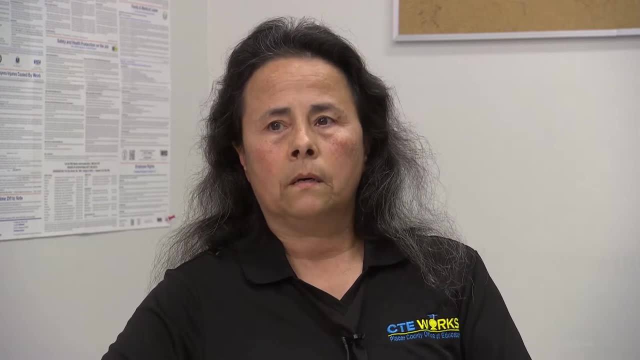 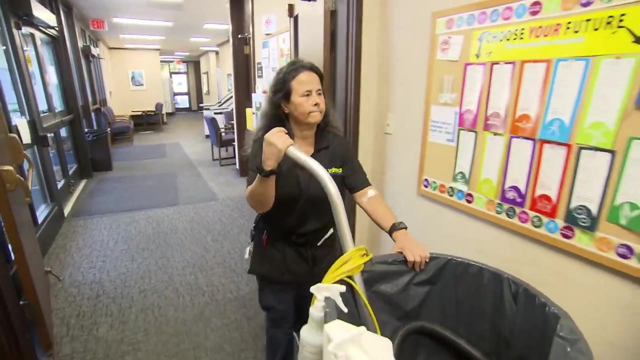 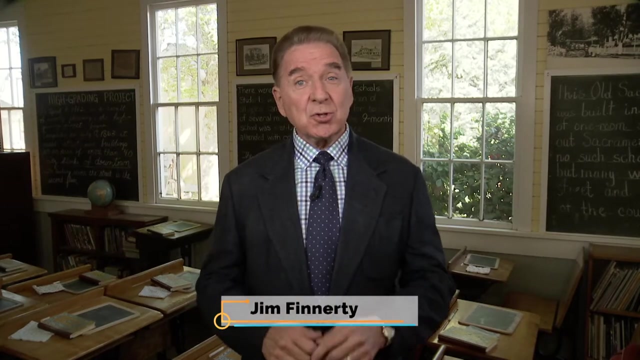 staff come in, it's clean, it's a joy to be here, You know they come in and it smells good, you know, And I get gratification that every day my job is done. And finally, let's visit two schools in Northern California that offer a learning program called 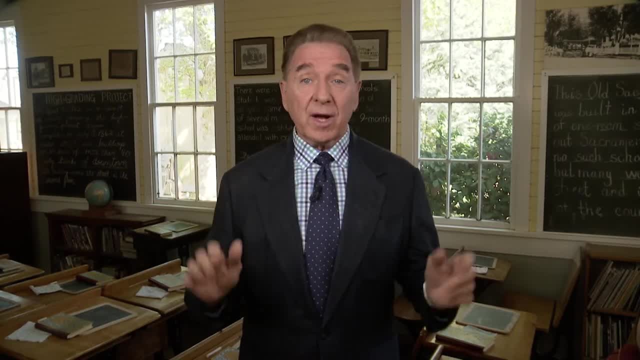 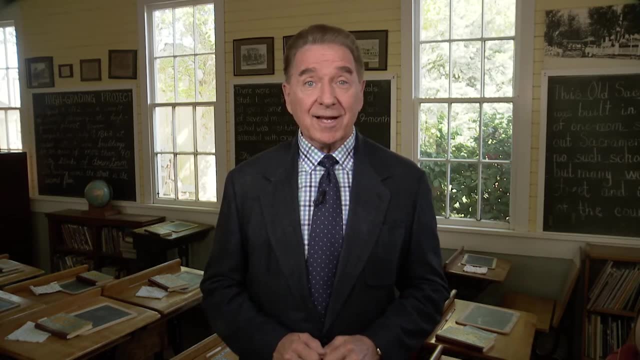 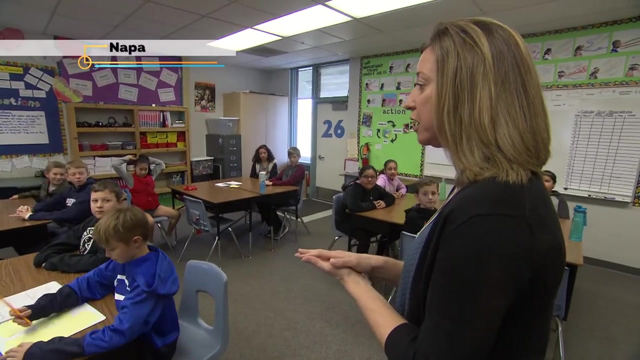 International Baccalaureate. You'll find them in schools all around the world. Let's discover how the curriculum works and why more students and parents are seeking out this style of learning. All right, fifth graders, if you could take your articles that you've been reviewing. 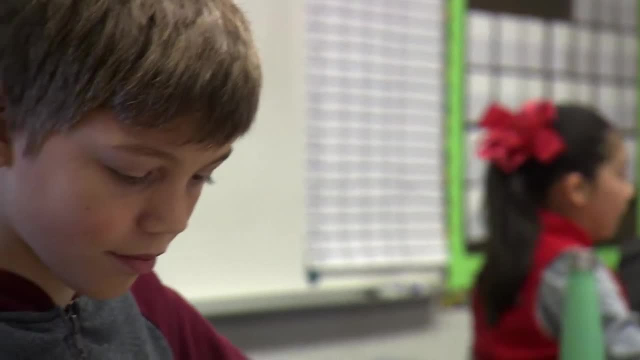 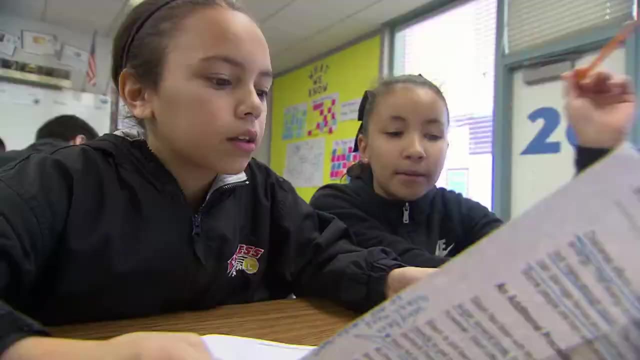 look through them and choose your five to six words that are most important. It's a typical morning in Leanna Alcayaga's class. Her students at Napa's Bel Air Park Magnet School are working in small teams, Reading, analyzing and discussing newspaper articles. 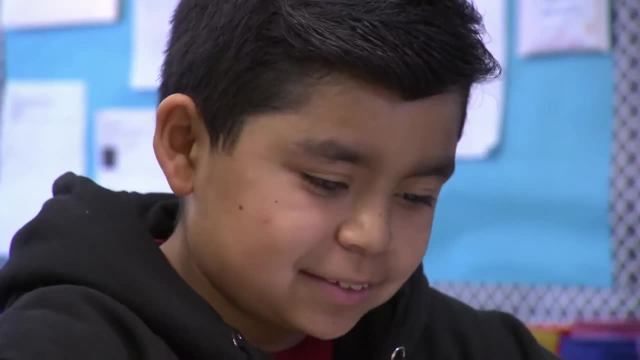 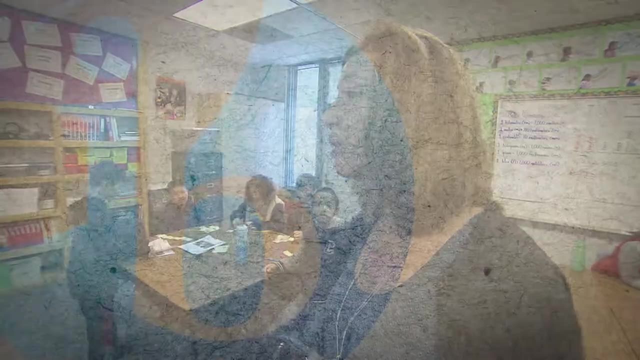 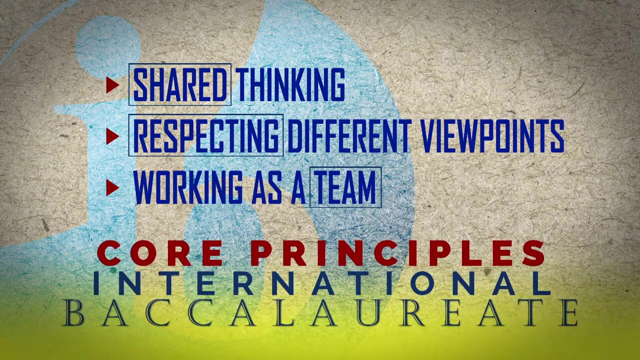 The conversations between these fourth and fifth graders are surprisingly thoughtful and thorough. Remember to be respectful when talking to each other and share your thinking. Shared thinking, respecting different viewpoints, working as a team: they're all core principles of the International Baccalaureate program. 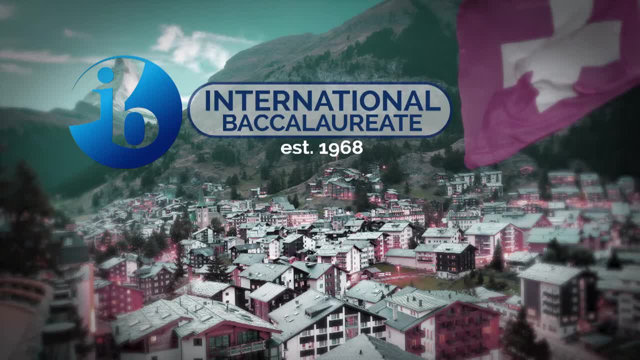 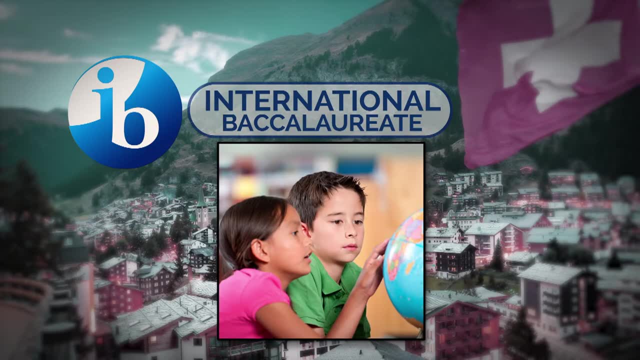 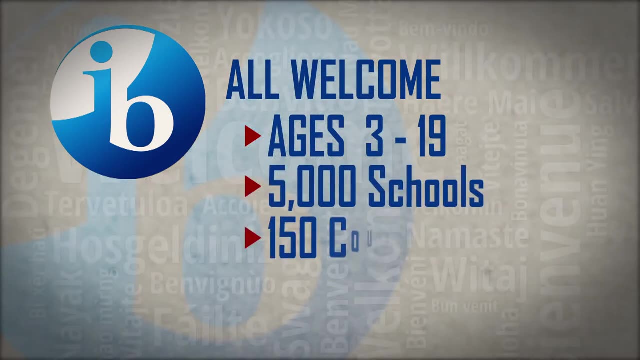 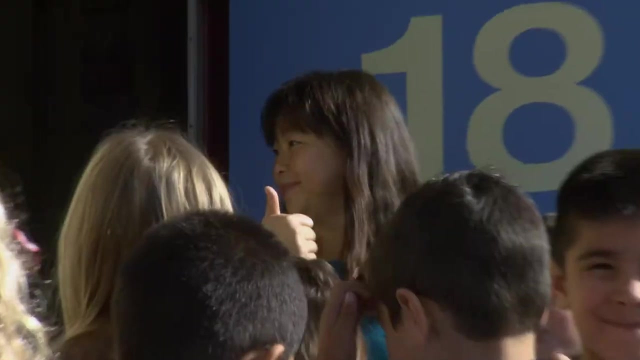 A nonprofit organization started in Switzerland in 1968, IB, as it's called, was originally designed for the children of diplomats. Today, it's available for any students aged 3 to 19, and you'll find it in 5,000 schools in 150 countries, with more than 900 in the US. 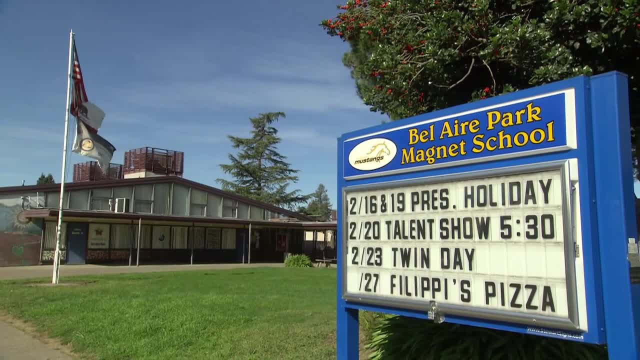 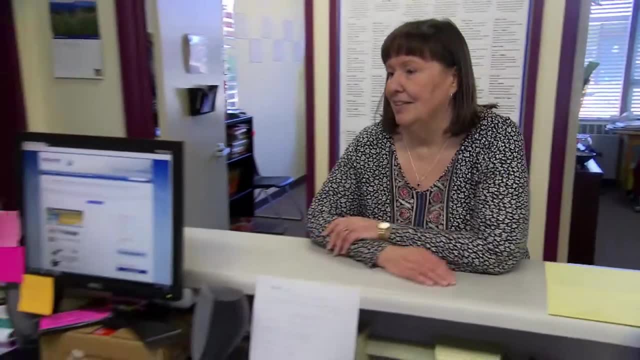 In 2009,, Bel Air Park became one of two IB schools in Napa, thanks in part to a federal magnet grant and thanks, says Principal Janine Burt, to a receptive community. Janine Burt Principal IB School in Napa. 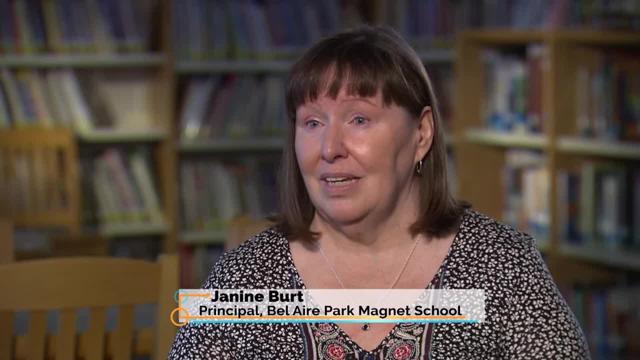 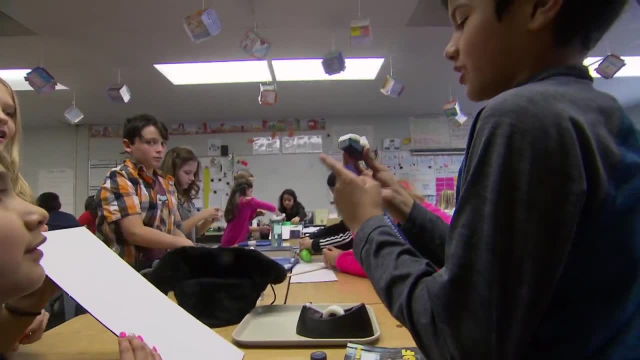 We're focused on how can we help every student that we see to become what they can become, and that's kind of the driving force behind it is that we have a purpose. Try several sliders, don't just try one. try three, four, five different ideas. 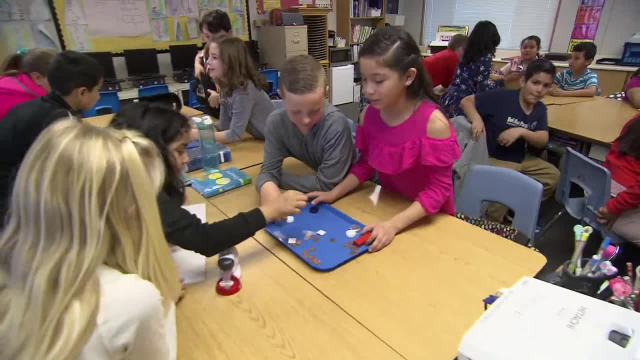 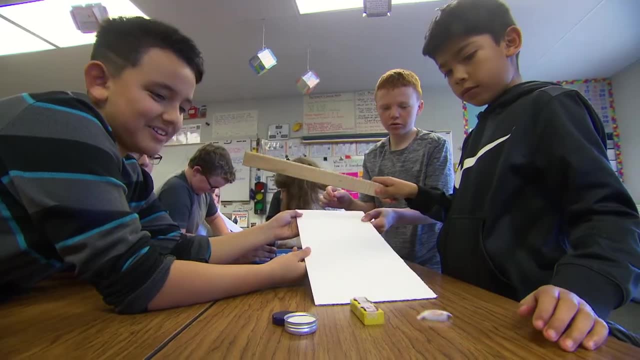 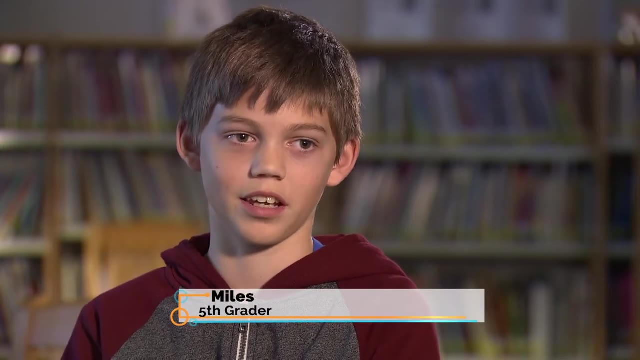 Over in Andy Terup's class. the kids are doing kinetic energy, gravity and friction experiments. Andy's provided some initial instructions but, like many IB classes, most of the learning here is self-directed and very interactive, Instead of the teacher just standing up and telling us to memorize dates and then naming. 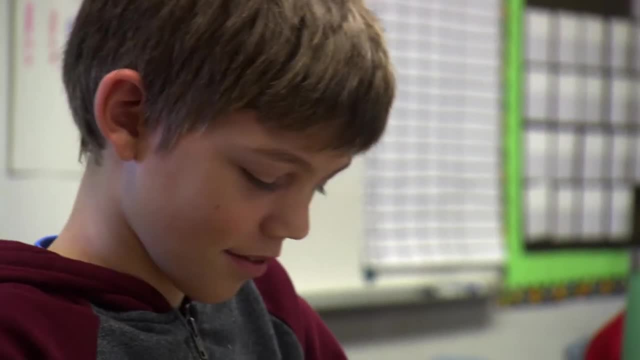 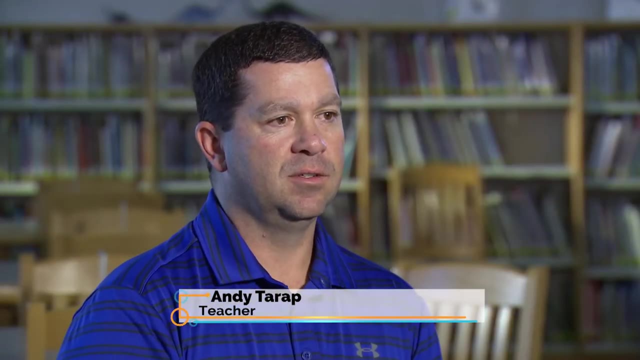 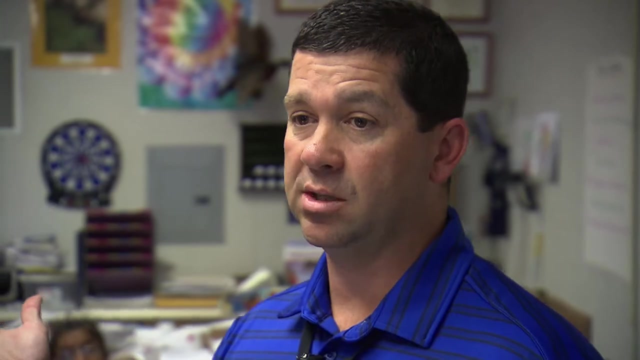 a bunch of dates for us to write down. we do like projects and we learn about different things. Coming from traditional class, it was very teacher-centered, very teacher-directed, Whereas now kids are really engaged. they're really talking about great things doing good. 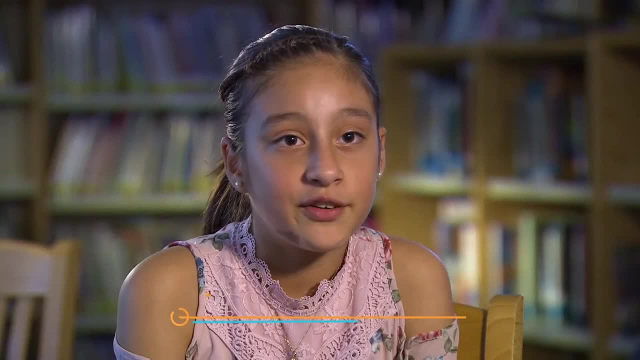 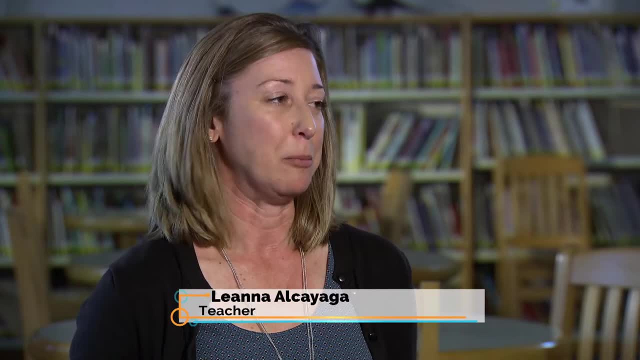 It's fun, It's fun, It's fun. We do a lot of good things because we do a lot of interesting things. I get really excited when they see that. It makes me want to call people and come in and see what they're doing, because it's not. 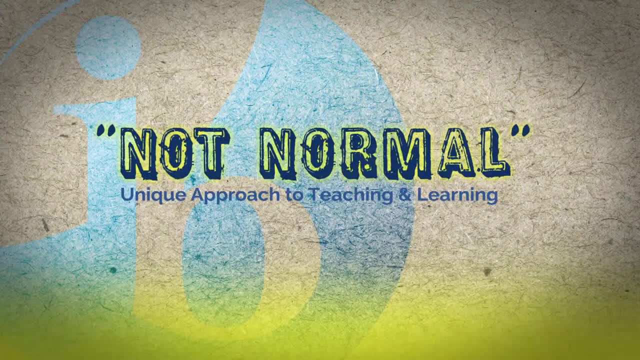 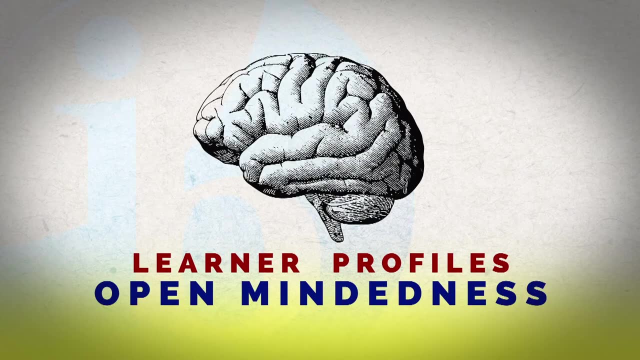 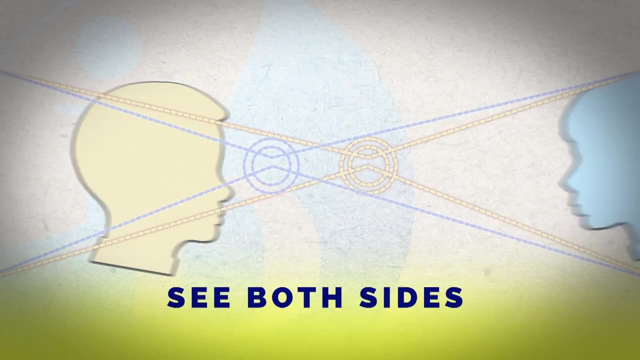 something normal. This not-normal and unique approach to teaching and learning is part of the IB goal to develop so-called learner profiles emphasizing inquiry, open-mindedness, independent and critical thinking, reflection, empathy and respectful communication. Students are encouraged to see both sides. 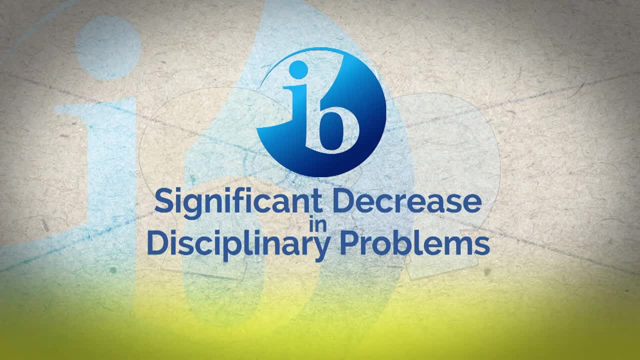 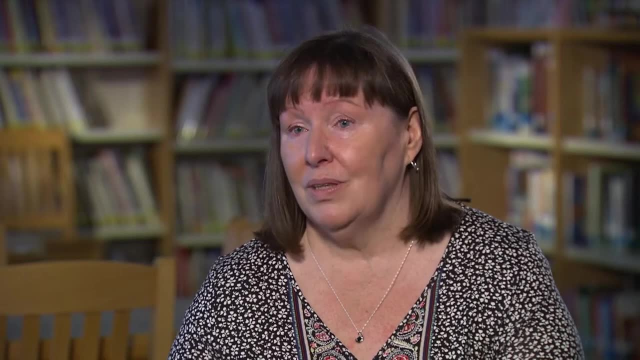 and respect others and their opinions. The result is often a significant decrease in disciplinary problems. If they're excited about what they're doing, they don't have time to have problems with other kids. They are, they want to learn, they want to be focused. 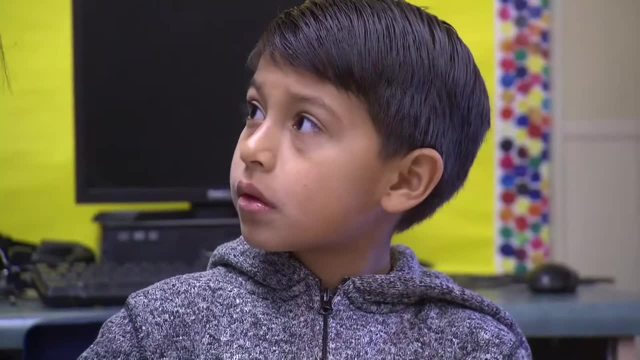 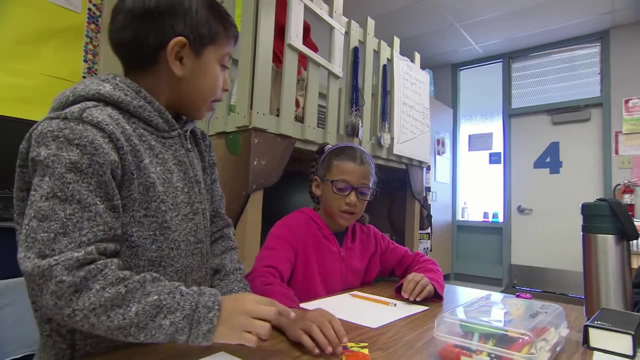 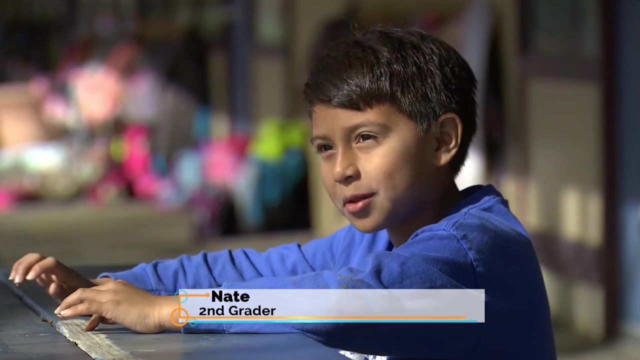 and they don't have problems because they're busy. The IB primary years program at Bel Air Park begins with very young students In this theory of knowledge. class second graders like Nate are studying artists from around the world. I'll feel excited because I'm learning about other people. 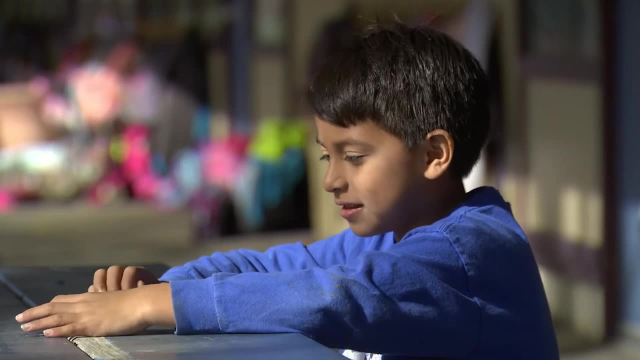 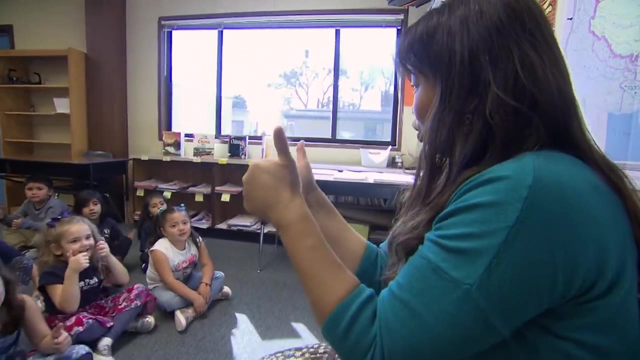 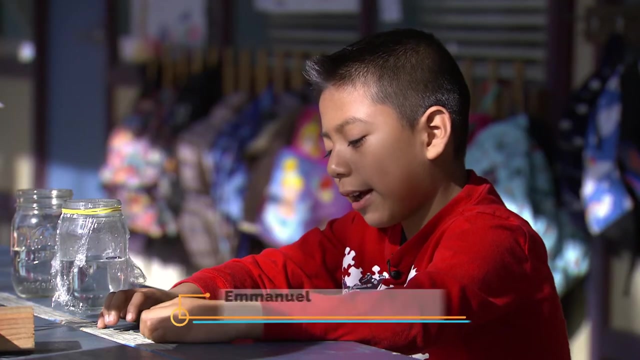 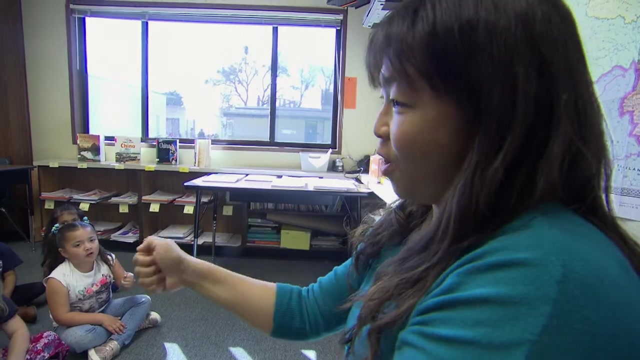 like the languages and like artists and like stuff like that. This second grade class is already starting to become fluent in another language. When I'm in fifth grade and I finally am done with Mandarin, I'm gonna know a lot about Mandarin. Students can remain in the program. 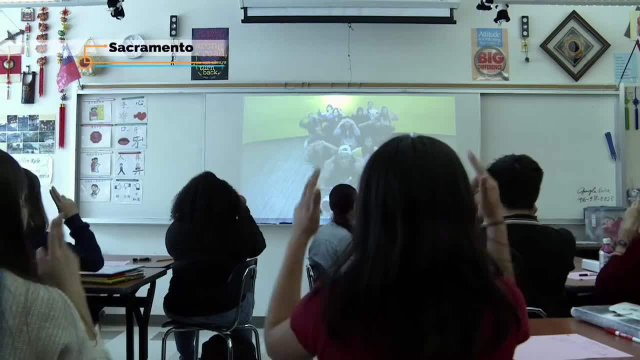 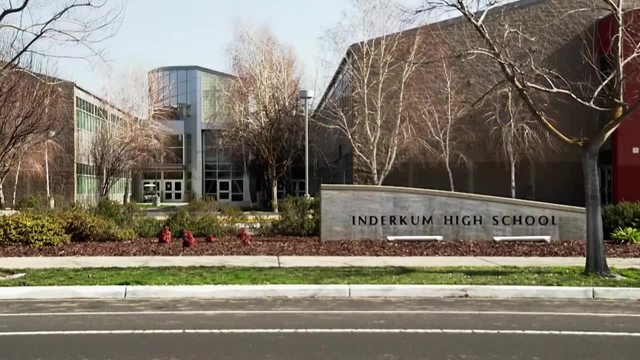 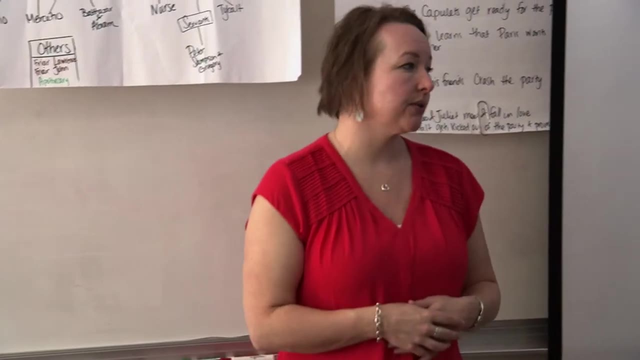 throughout their K-12 academic career. Sacramento's Intercom High School has been an IB school since 2014 and graduated its first class two years later. Some of its teachers, like Karen Taylor, have taught IB classes in such far-flung places. 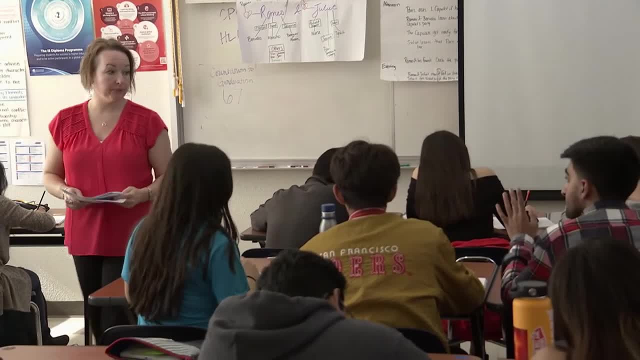 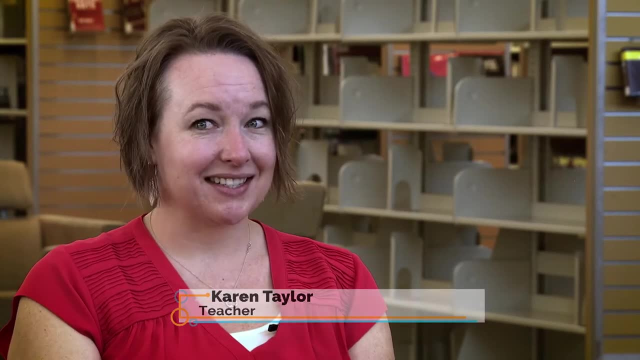 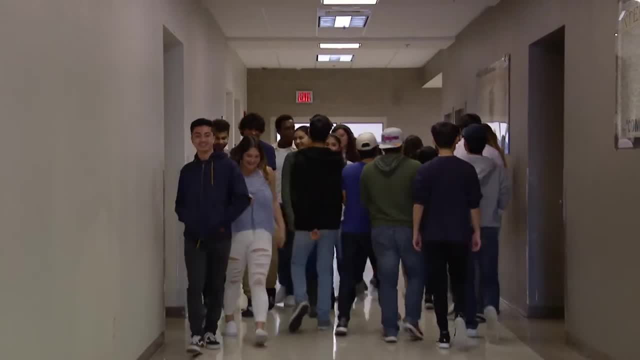 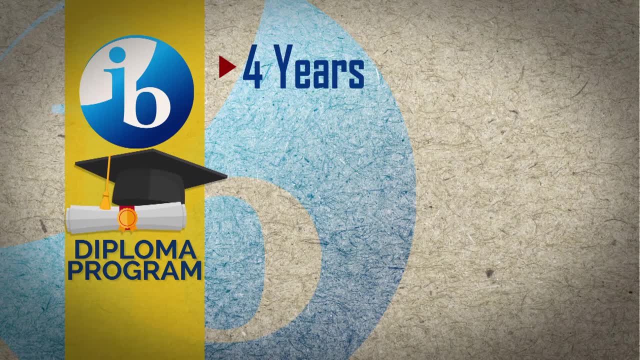 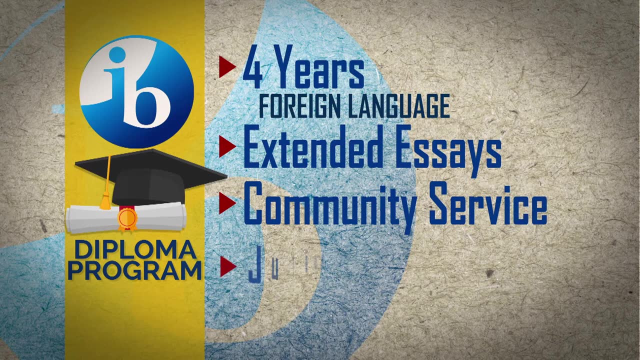 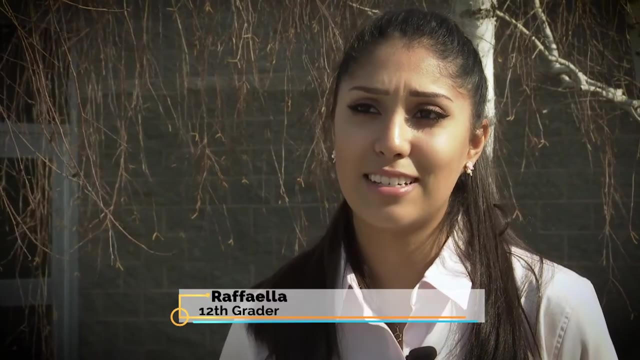 Many of these students are taking part in the diploma program, which requires four years of foreign-language study, writing extended research essays, a community service project, even junior and senior exams judged by IB experts around the world, And so it really gives you a good practice. 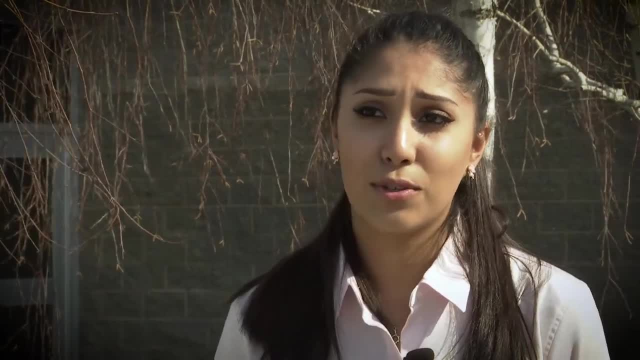 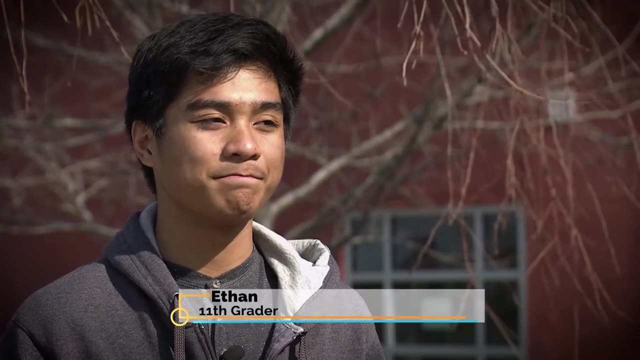 to make it a lot more easier process for you so you can be successful in college too. Just the rigorous amount of work that we're being given here and how we're being trained to really manage our time well is going to prepare us really well for college, because 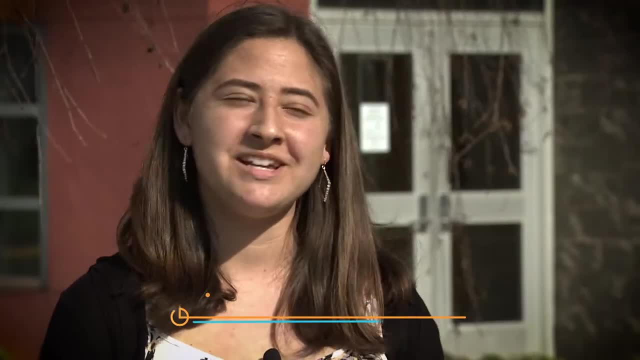 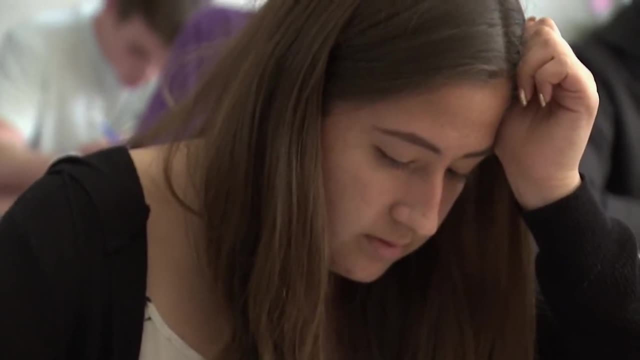 we're going to have a lot of work and very little time. If you're looking for an easy way out, this definitely isn't. It's very rigorous, but it's so rewarding. Among those rewards, students earn points that can be translated into quarter and semester. 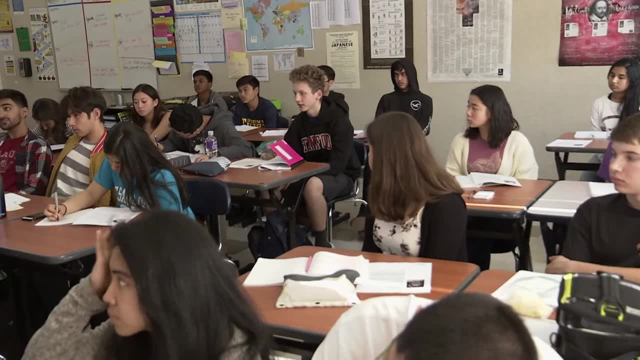 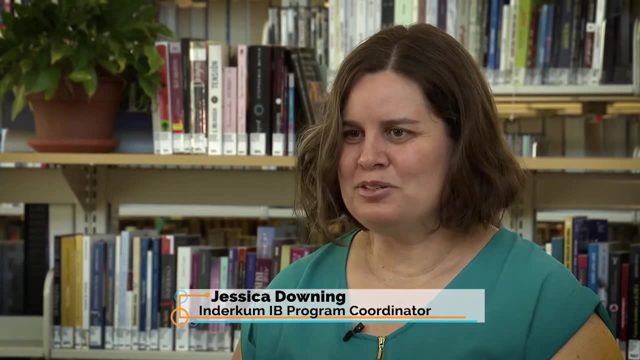 credits at the University of California and recognized at many other colleges worldwide. The IB diploma would be recognized in so many more places, whereas no one necessarily knows where Indicom or Sacramento is. but they understand what an IB diploma is, and so that's a credential they can carry forward with them. 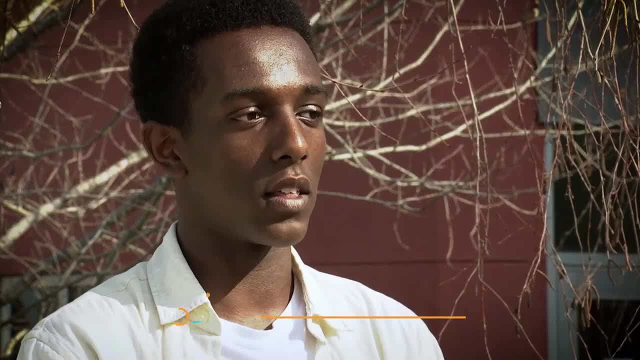 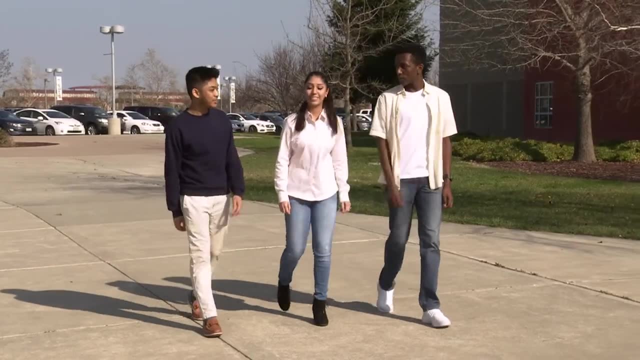 Looking back on all the years of the IB and my experience within it, I think that I wouldn't be half as capable as I am today if I had not participated in the program. Schools must pay a fee to join the International Baccalaureate and many say it doesn't just. 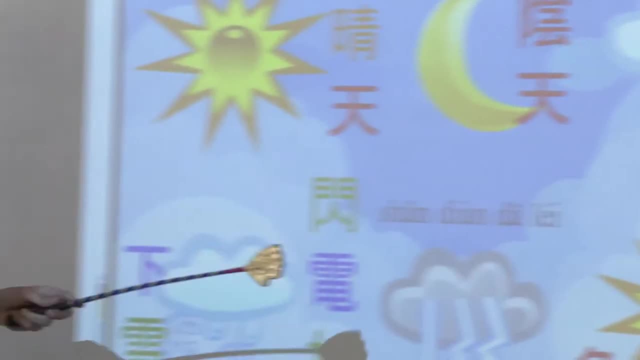 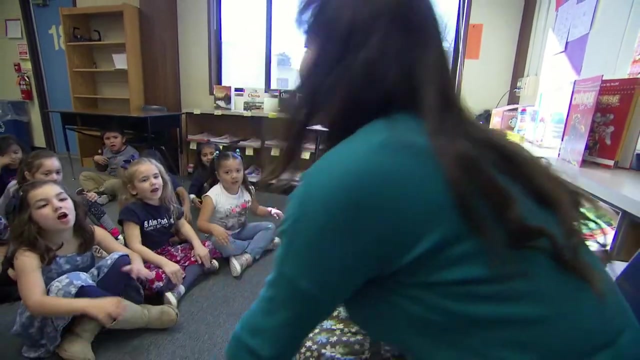 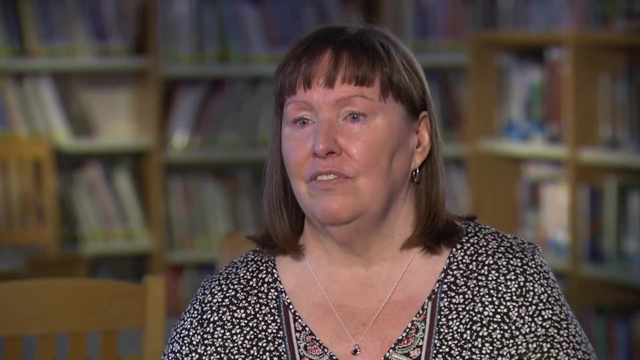 require hard work, but often a fundamental change in thinking about the student-teacher relationship, What education should be all about and how to use knowledge to help make these young people true global citizens. It just creates this environment where it feels like learning is fun. it feels like 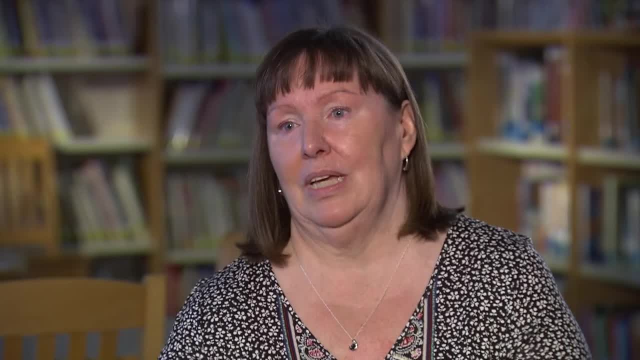 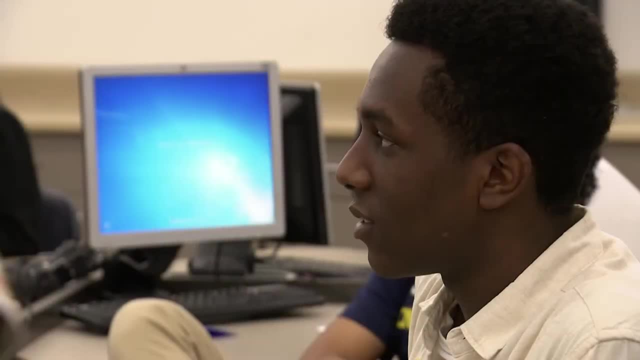 learning is important and they're doing it. I can't even imagine going back to a traditional school and teaching. I love my classes and my teachers, and I think that it's a good fit for people who are dedicated to their education and to making the world a better place. 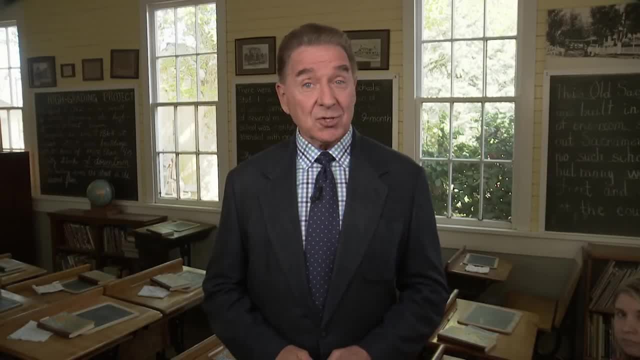 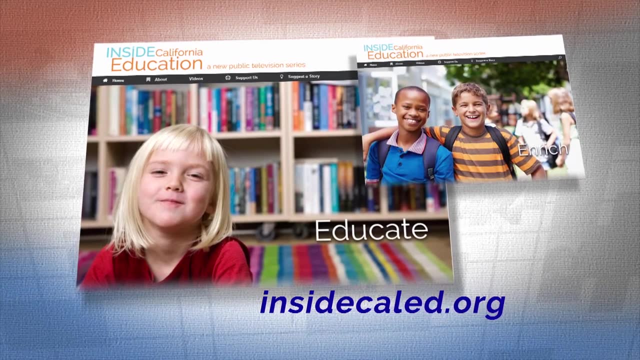 That's it for this edition of Inside California Education Now. if you'd like more information about the program, just log on to our website, InsideCalEdorg. We have videos from all of our shows and you can connect with us on social media as. 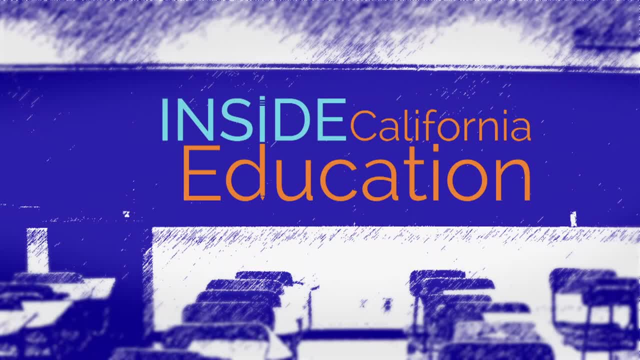 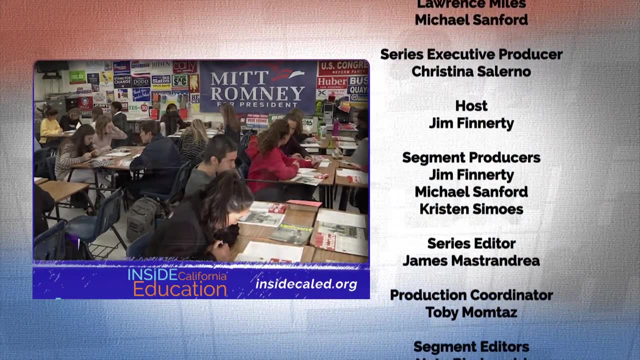 well, Thanks for joining us. We'll see you next time on Inside California Education. Okay, so I'm going to give you until 10 after to read this article and take notes on it. As a student, I believe there should be no tuition. I'm going to give you until 10 after to read this article and take notes on it. As a student, I believe there should be no tuition. I'm going to give you until 10 after to read this article and take notes on it. 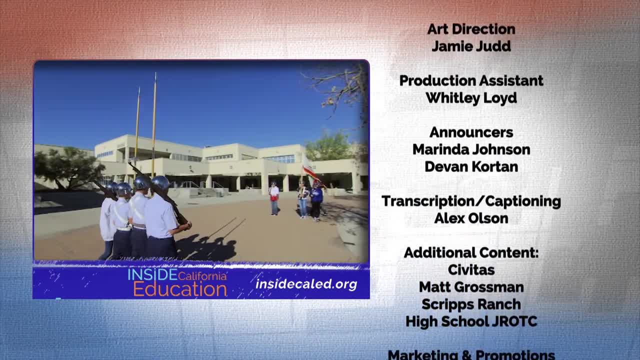 As a senior, I believe there should be no tuition. I'm going to give you until 10 after to read this article and take notes on it. I don't believe we're even going to have a tuition increase. Left, left, left, right turn.